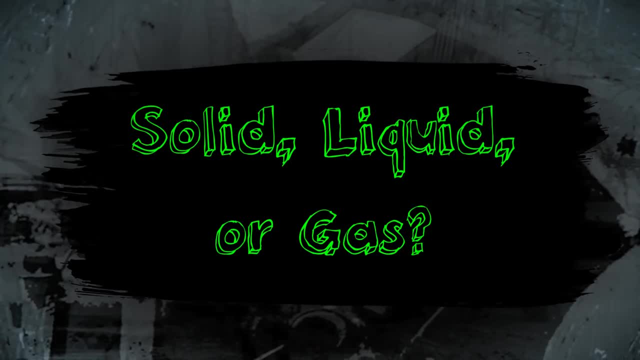 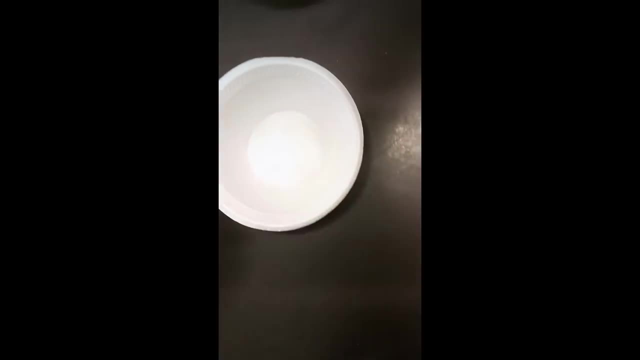 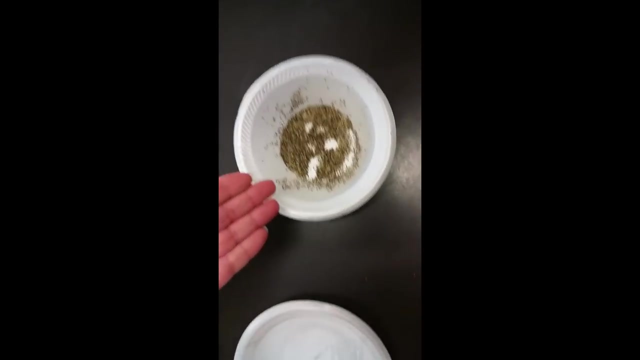 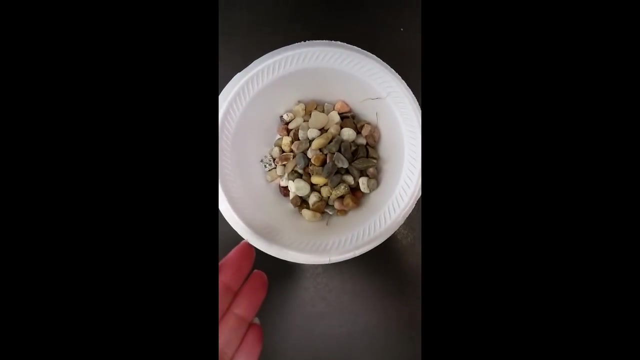 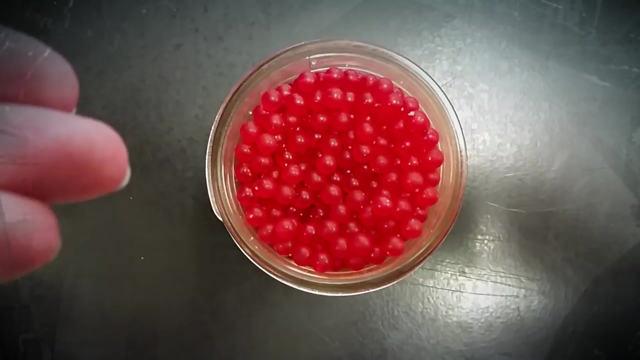 Here's the first one: Water. Next we have our salt right here. Next is pepper, We have some sand And then finally we have a bowl of small peppers or rocks. We are now on the second column of our paper. At the very top, you'll see that this first one is plastic beads. Now we have 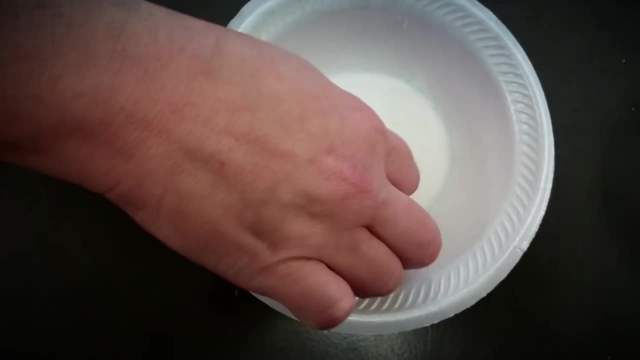 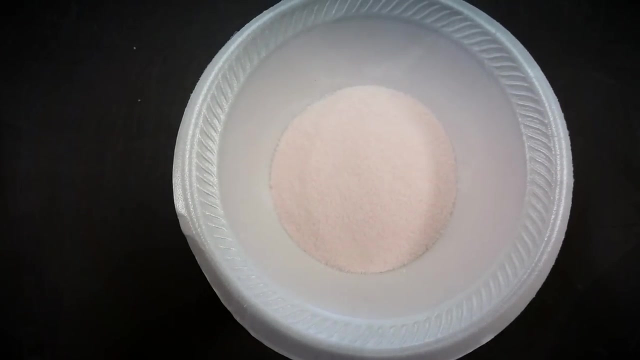 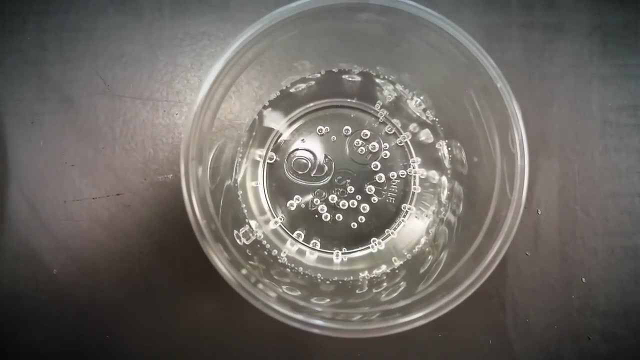 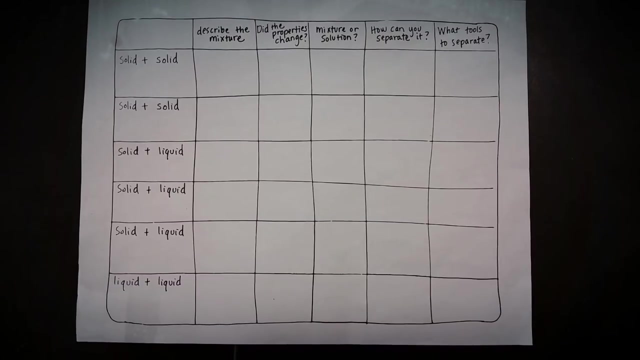 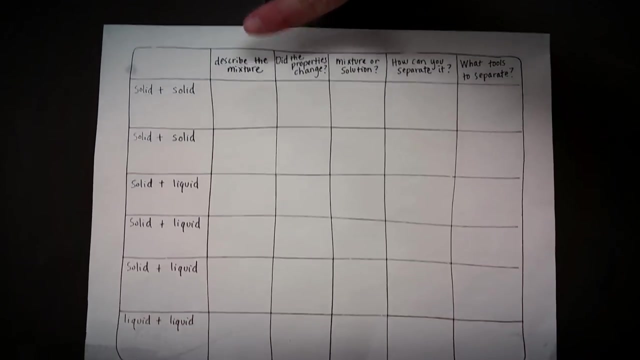 metal beads Sugar. This is a drink mix like a Kool-Aid mix And lastly, we have some Sprite soda. On the back side of your paper you will see this chart. We're going to be filling in each column, starting with: 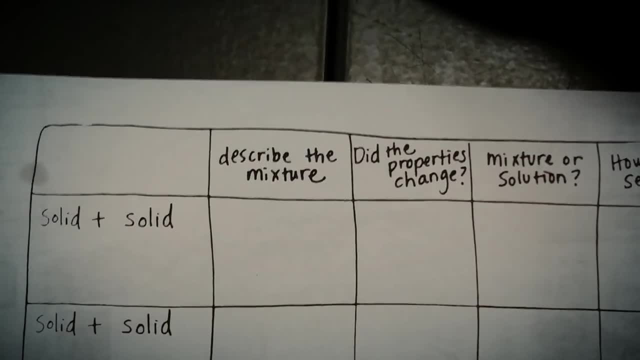 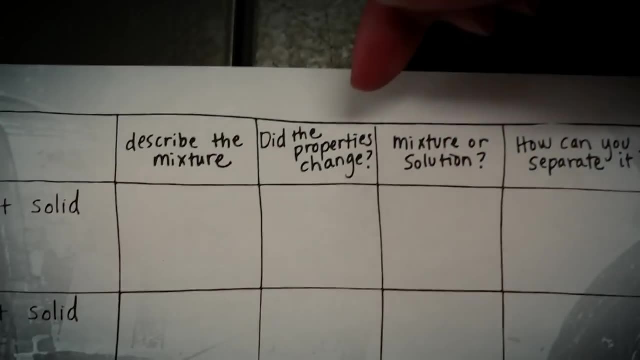 describe the mixture. So when we pick our items, we're going to name what they are, For example, sugar and salt. if that's our mixture, Our next column is going to be: did the property change? So we're going to decide. 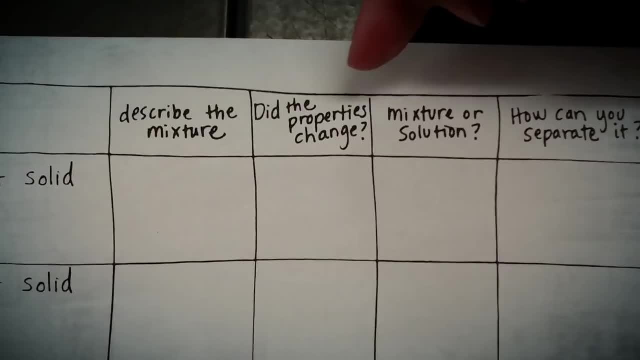 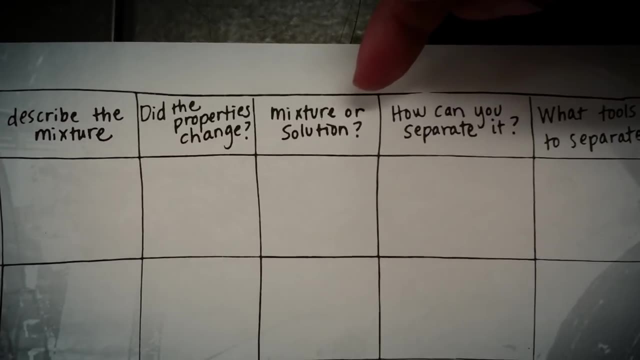 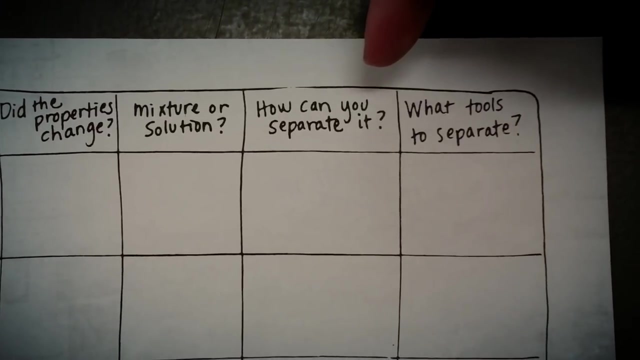 yes or no on whether the properties have changed once they've been mixed. Mixtures and mixture or solution. if that is exactly what we're going to put, is it a mixture or is it a solution? how can you separate it? so we're going to decide what process to use to separate it and remember: 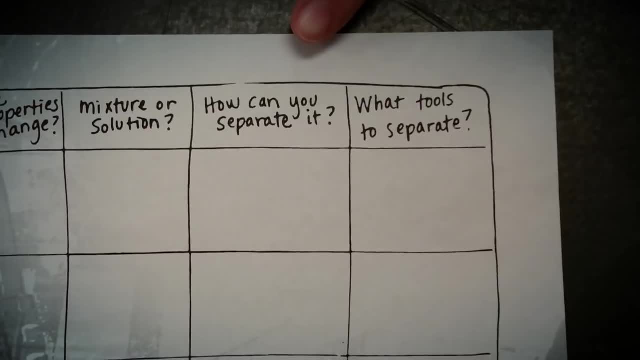 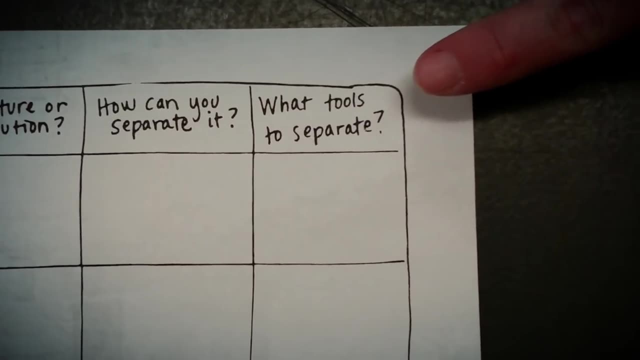 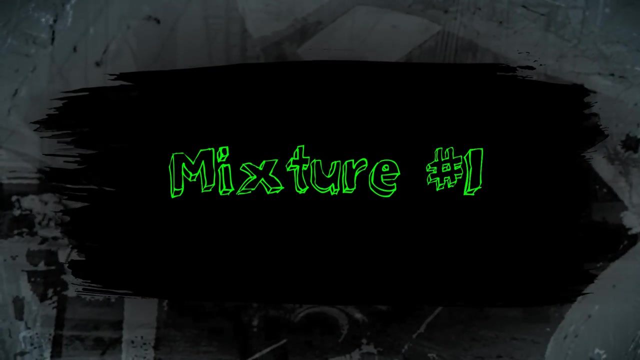 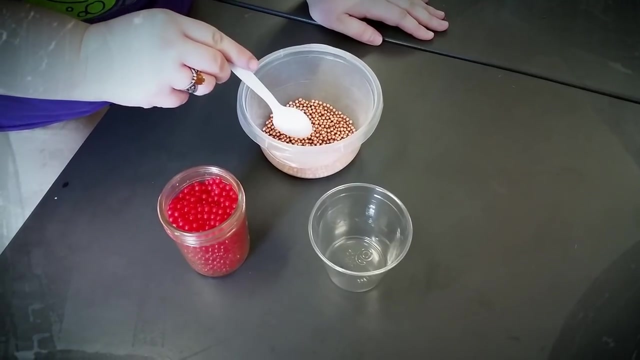 with separating. if it is dissolved, are we able to separate it? okay, and then our final column is: what tools to separate? so what are the tools that we're going to use for this process? so in our first column, in our first row, we're going to mix together some metal beads and some. 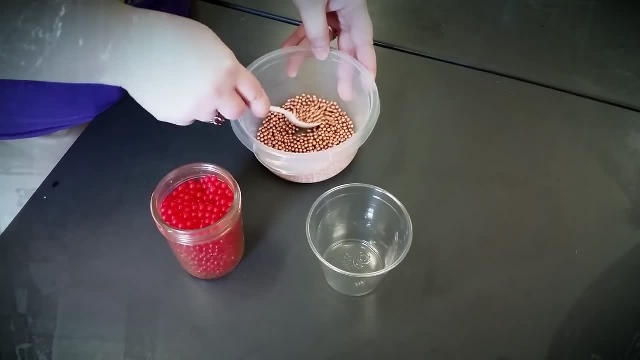 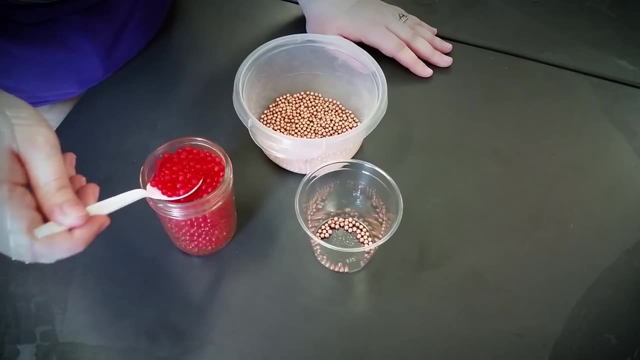 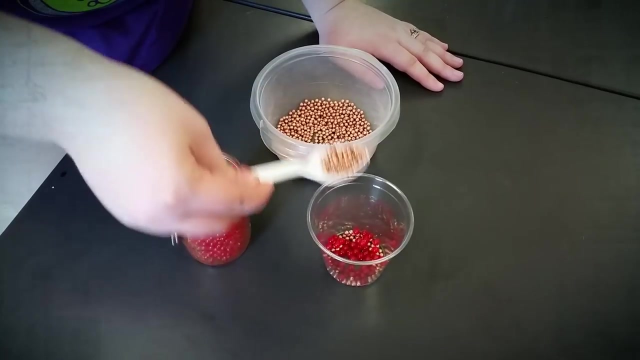 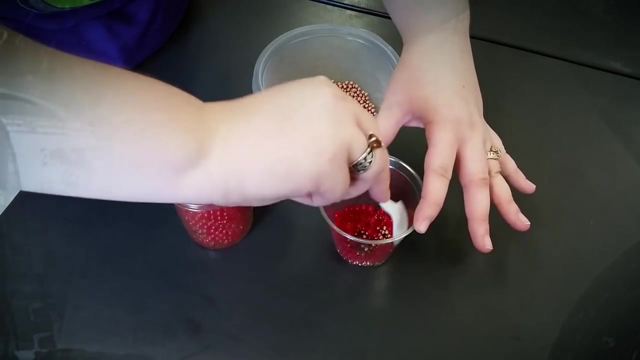 plastic beads, and i'll take a shoot here while i'm doing this. you can go ahead and write metal beads and plastic beads in your description. just do a couple of shoots here. all right, now we're going to write under. did the properties change? i've mixed it together, i want. 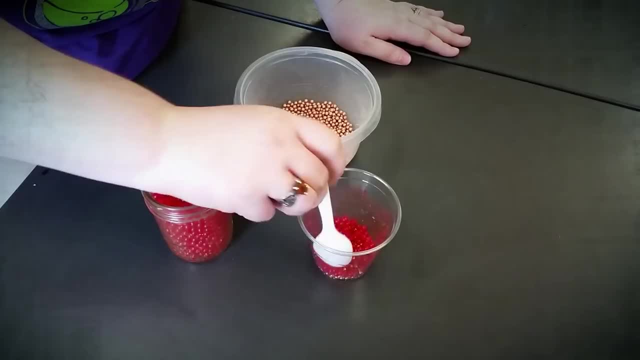 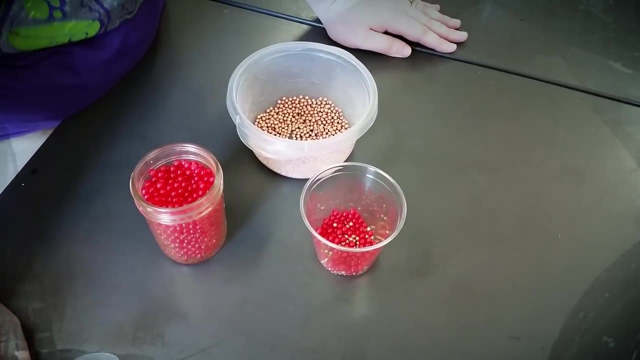 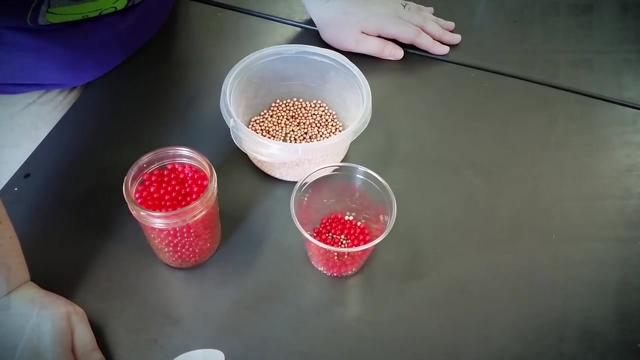 you to decide: has anything about these changed? are they still a solid liquid or gas, or has something changed? in the third column, i want you to decide: has anything about these changed? are they still a solid liquid or gas, or has something changed? anything dissolved? is it a mixture or a solution? 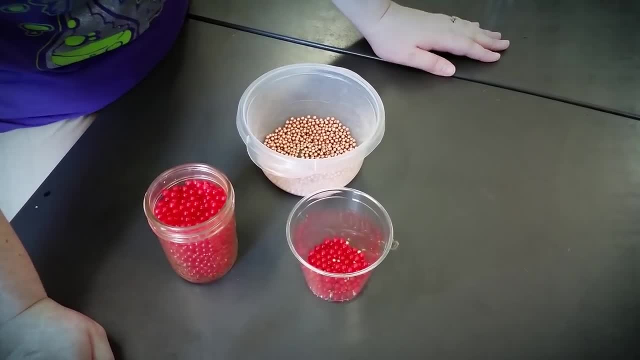 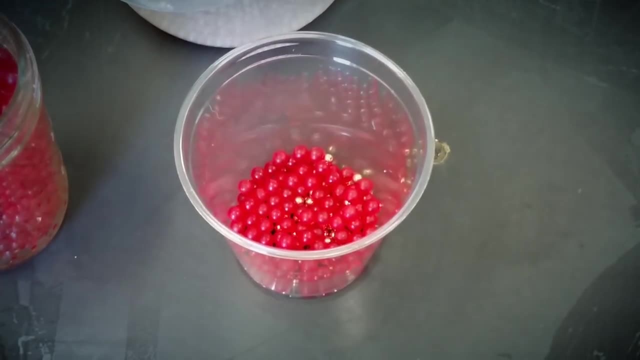 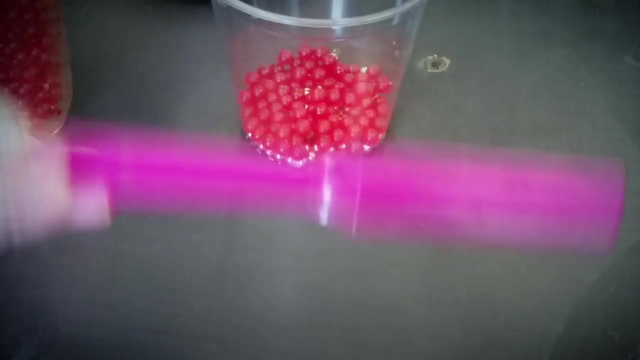 in the next column we're going to decide: can you separate it? i want you to take a guess. now, in the fifth column, we're going to say: which tool did we separate it with? i have with me today a magnet, magnets on the inside part, right here now. i have metal beads and i have plastic beads. 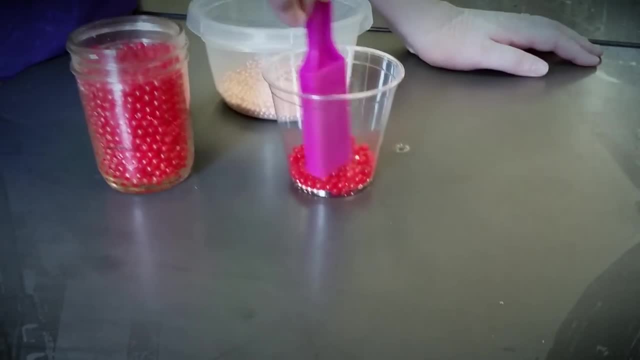 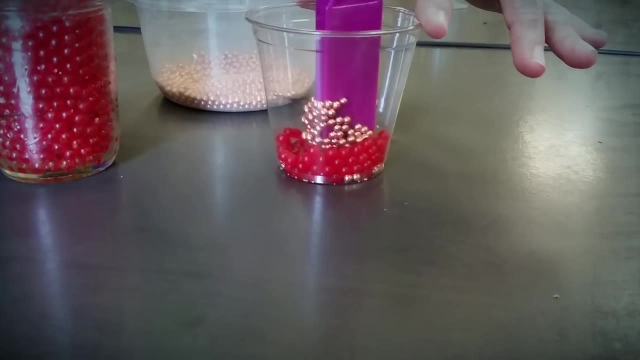 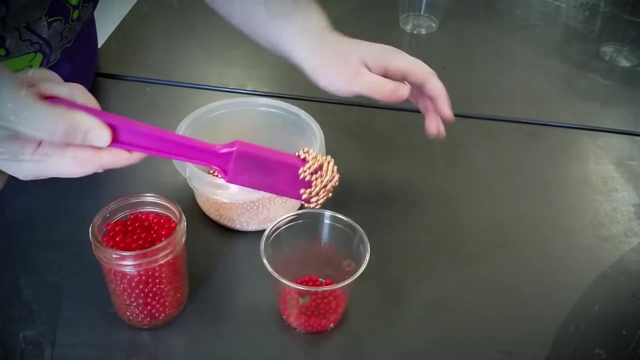 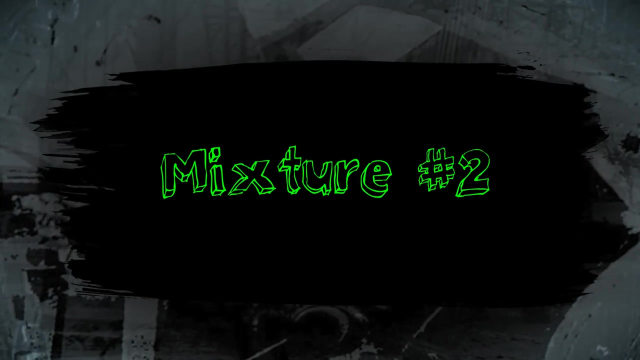 plastic, as we know, is not magnetic, so I am going to put this around, make sure I get the mold. And now I have the metal beads and the plastic beads For our second mixture. we are going to mix some rocks, small pebbles, with some sand. 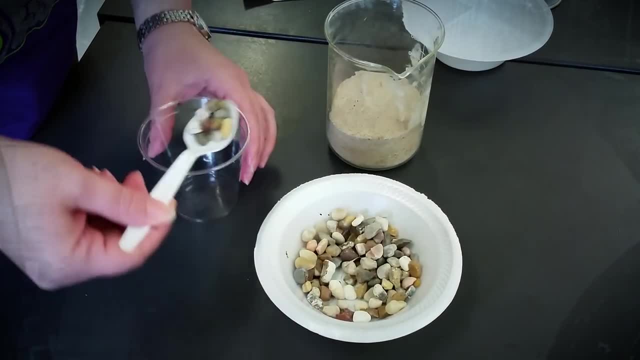 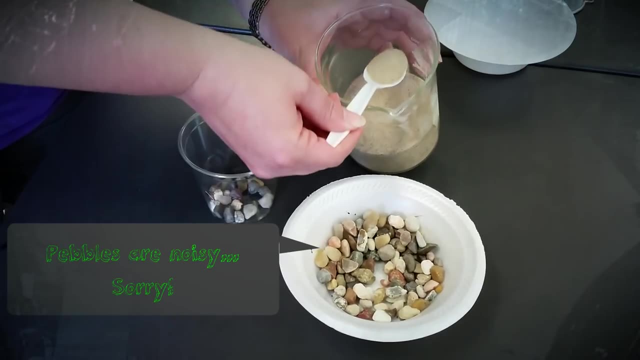 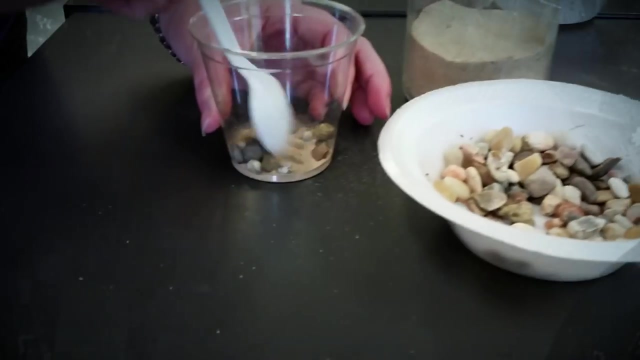 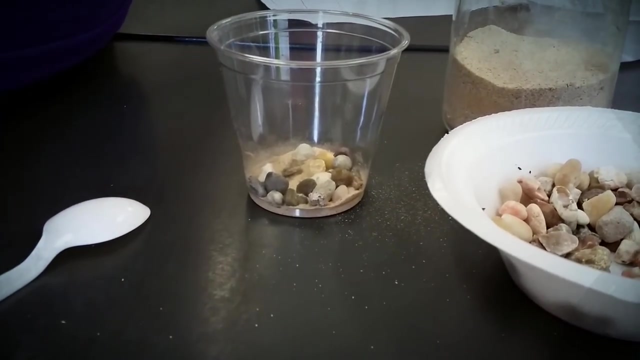 So I am going to take a few spoonfuls of rocks and then some sand and mix them up. So in our first column, describe our mixture. make sure that you write down your sand and your rocks. And then did the properties change in the second column? so, has anything changed? did? 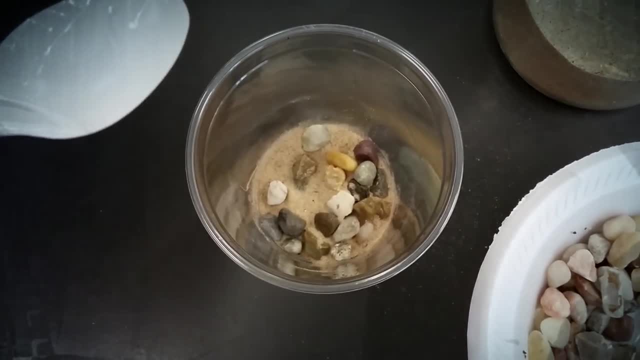 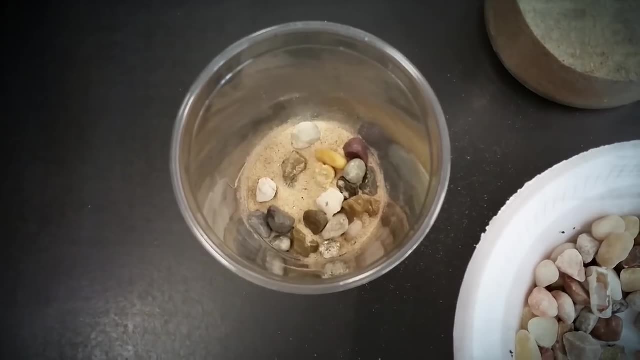 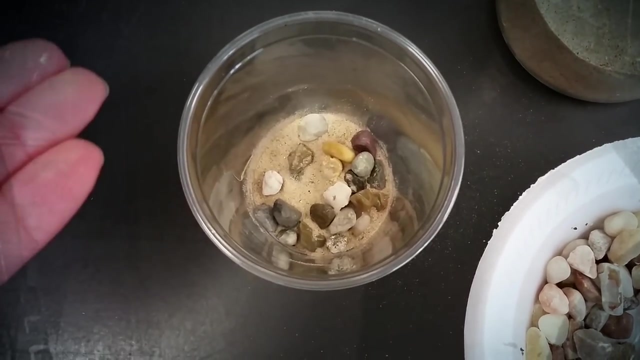 the rocks dissolve. did the sand dissolve? In our third column we are going to decide: is this a mixture or is this a solution? So now we want to try to separate it. so we are going to pick a tool that can separate the bigger rocks from the smaller sand. 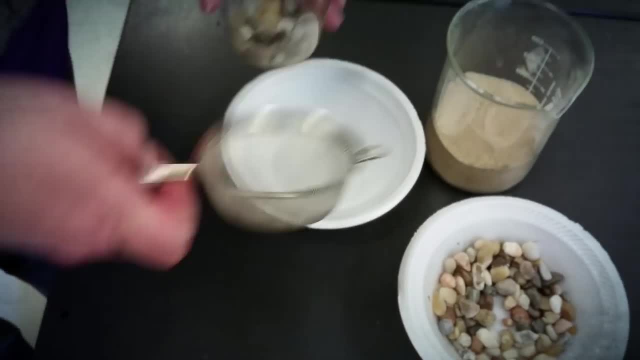 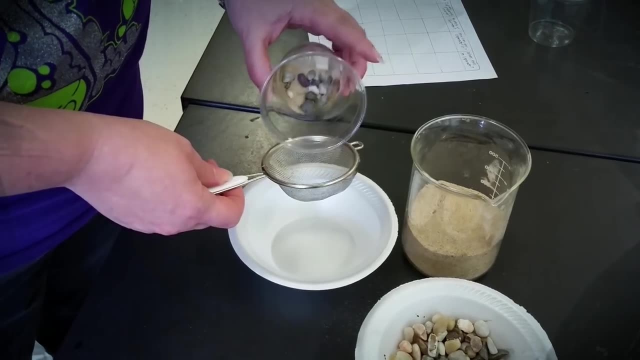 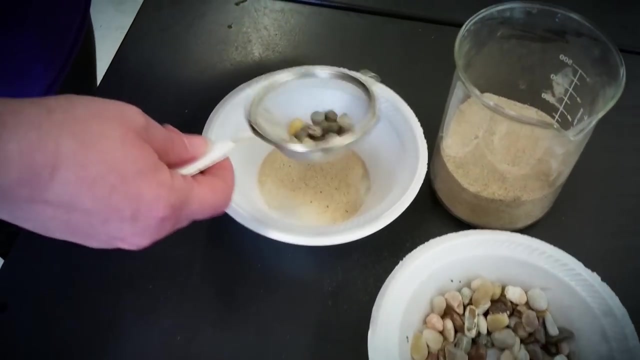 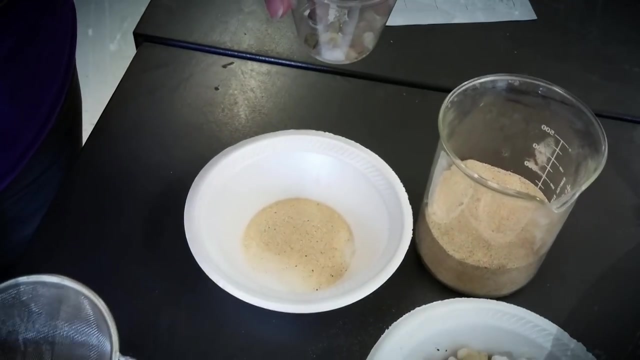 So I have another bowl here And I picked a strainer or a sieve to do that with, So I am going to pour the mixture into it, give it a little shake, and now you can see that the rocks are by themselves and the sand is now in the bowl. 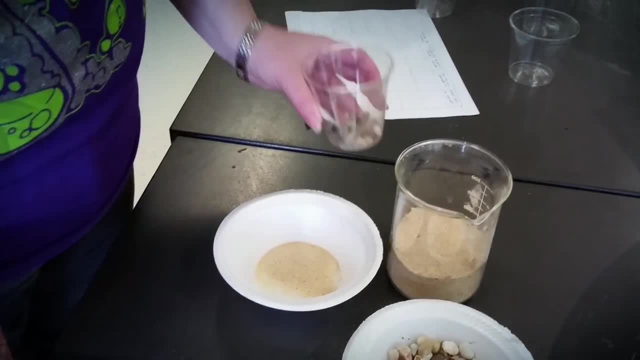 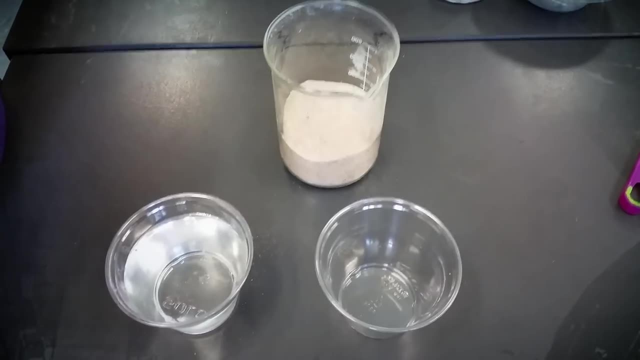 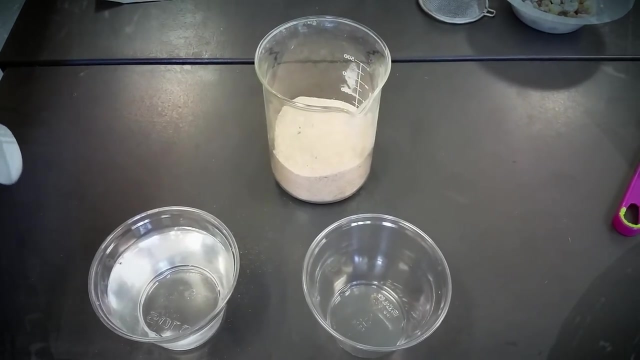 So we have separated them. We're now on our third row. It says solid and liquid. off to the left We're going to use sand as our solid and water as our liquid. So take this time to write down sand and water and describe the. 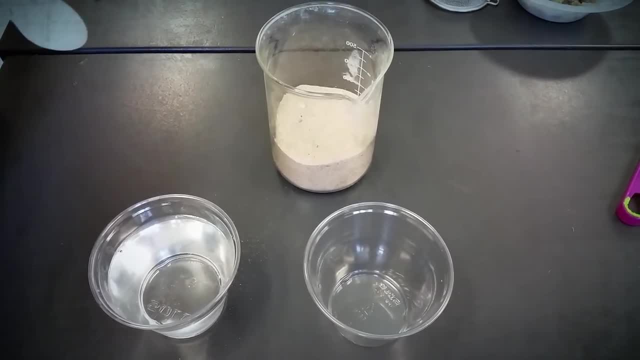 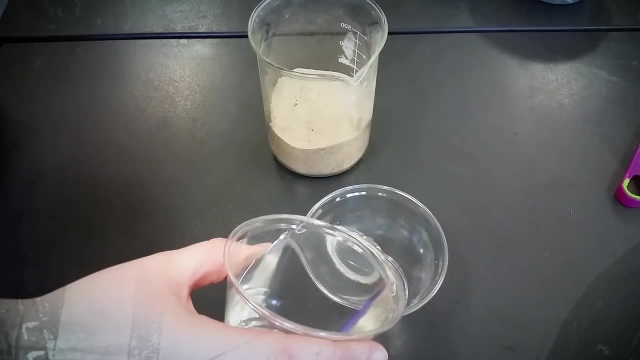 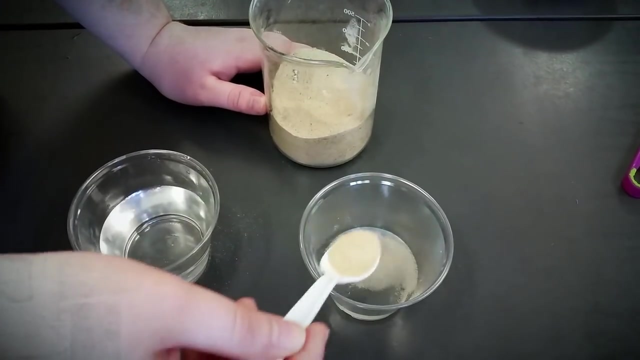 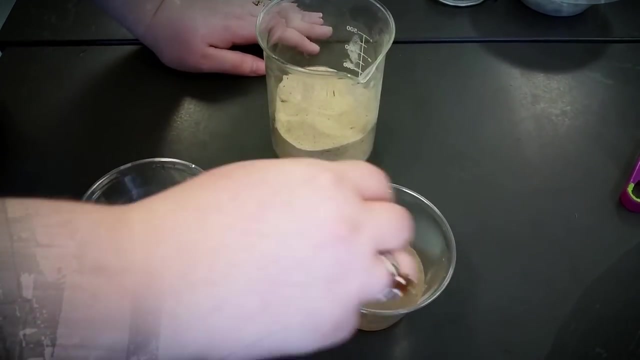 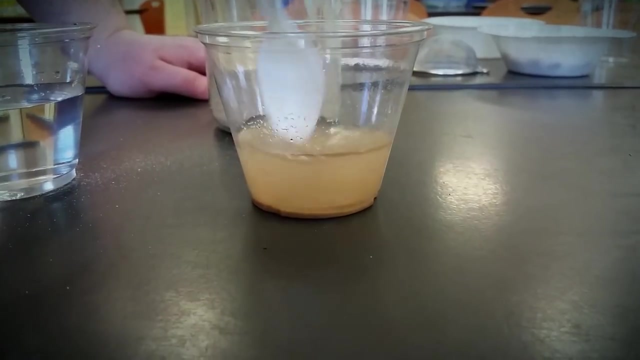 mixture We're also going to look at. did the properties change? So I'm going to go ahead and I'm going to pour a little bit of water in. I'm going to pour a little sand in, Mix it up. You can see that the water looks real murky. now I can feel with my spoon that it is very. 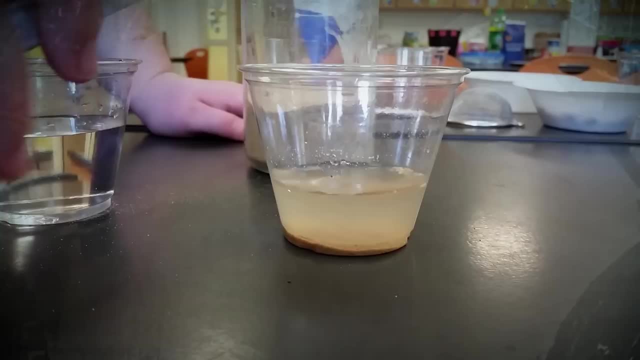 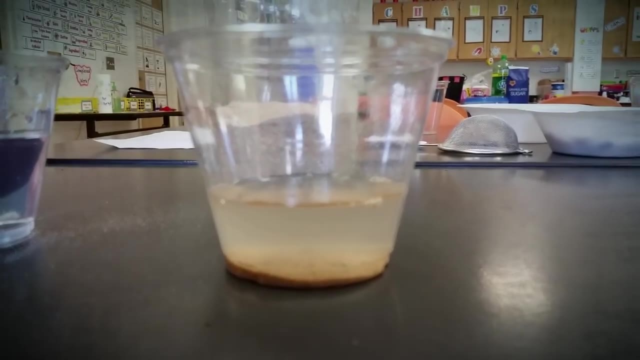 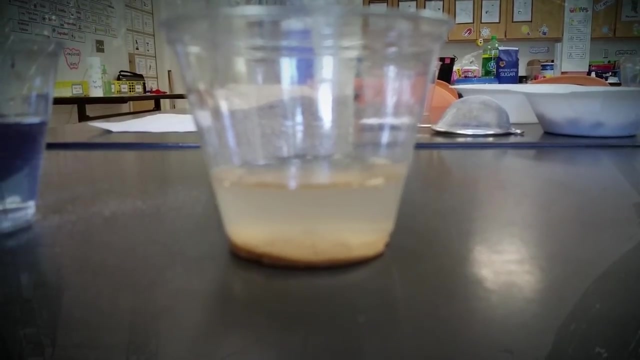 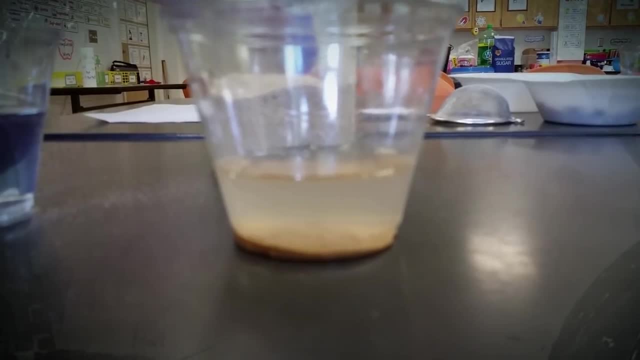 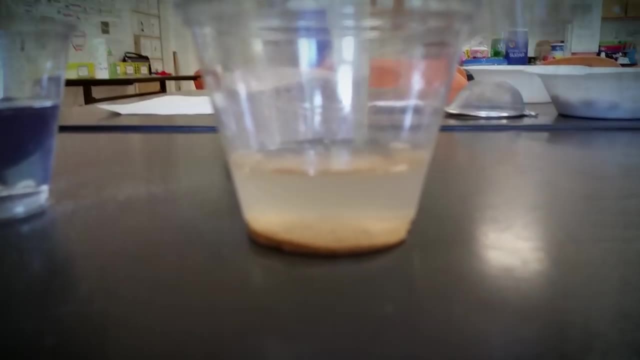 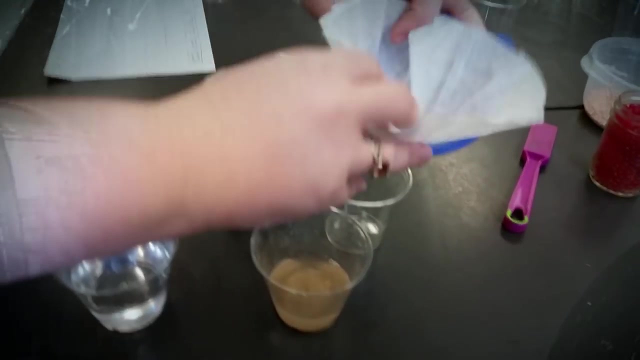 Now we're going to decide if we can separate it and what we're going to separate it with. I have a second cup. I'm gonna go ahead and use this funnel. I put a filter inside of it. It's just a coffee filter. You'll see, the filter is very 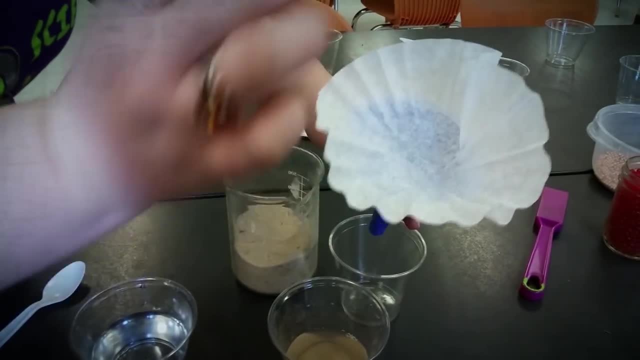 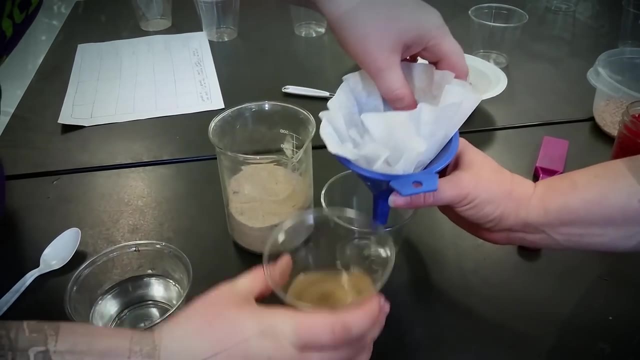 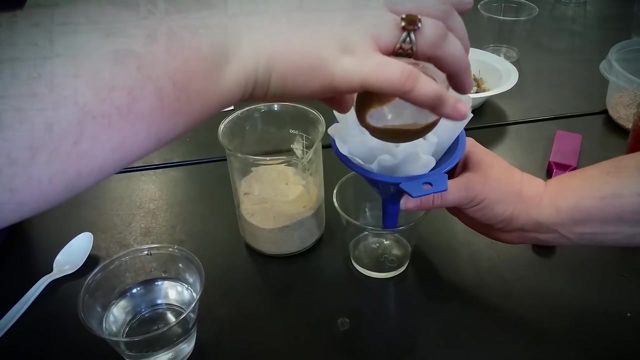 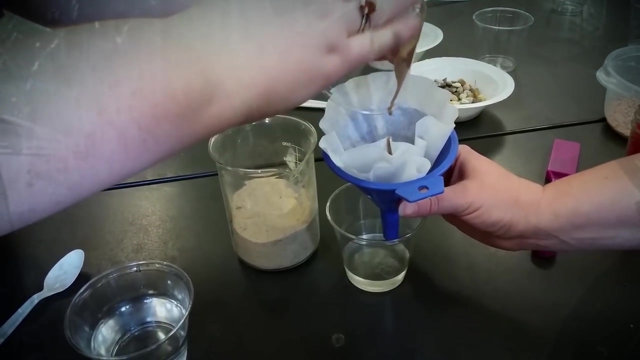 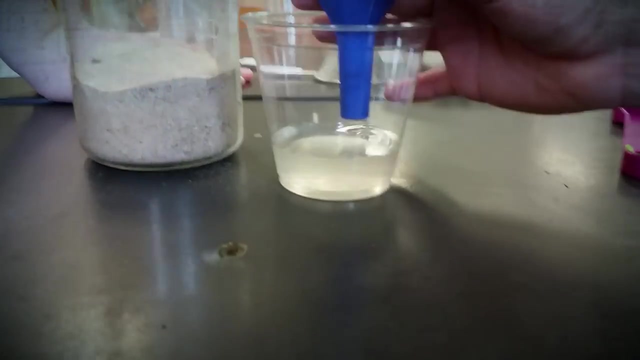 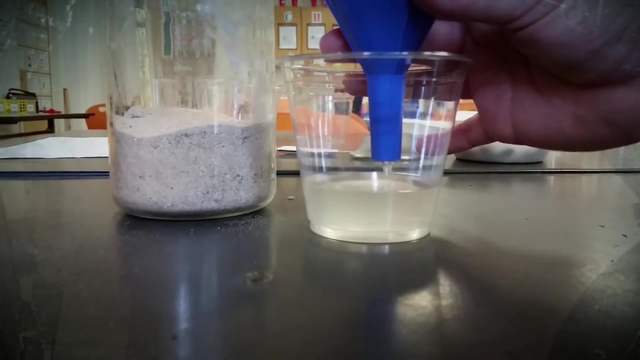 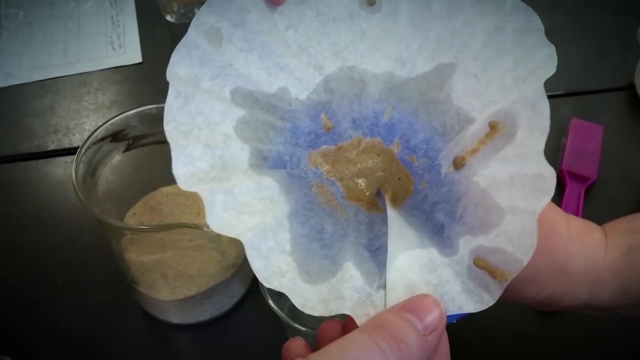 porous. so anything liquid is going to go through the filter and anything solid is going to be stuck. Pour this in here, And already my water is starting to pour through the filter. Let it drip. You may see in the filter. now we have sand in the filter and in the cup is just water. 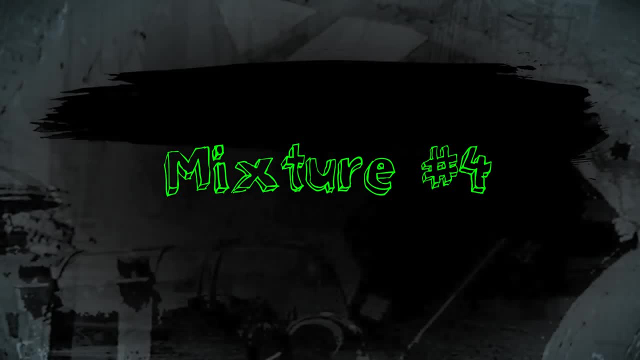 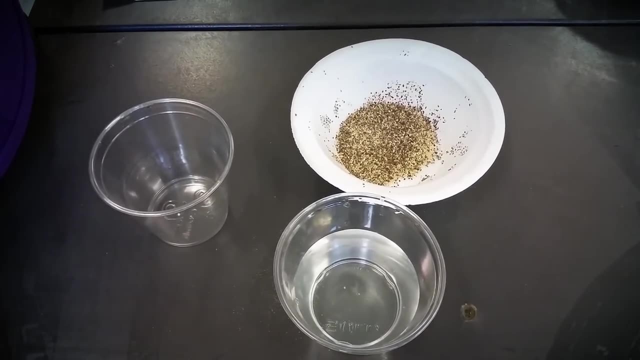 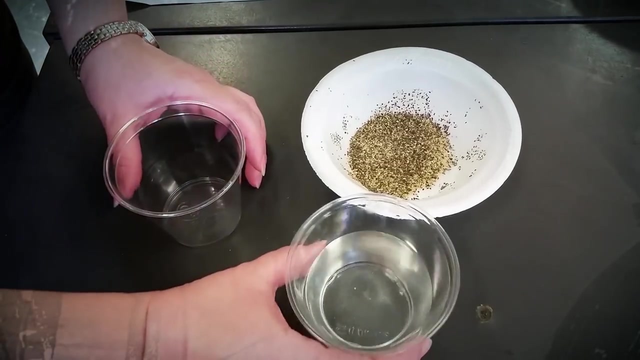 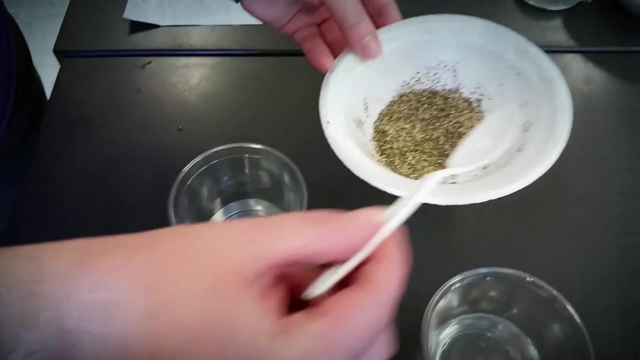 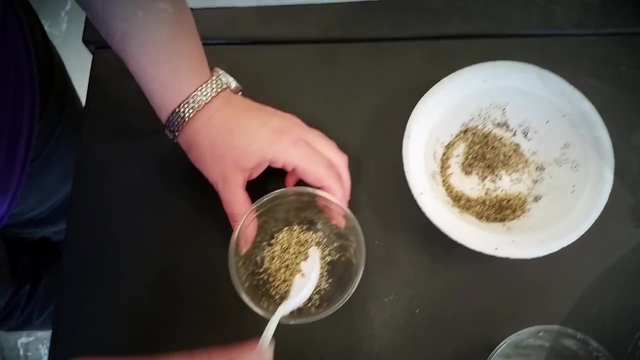 No more sand. on your fourth line you will see solid and a liquid again. so we're going to mix the water with the pepper this time. so I'm going to go ahead and pour some water to start with, and then I'm going to put some pepper in. go ahead and take a second to write that down. 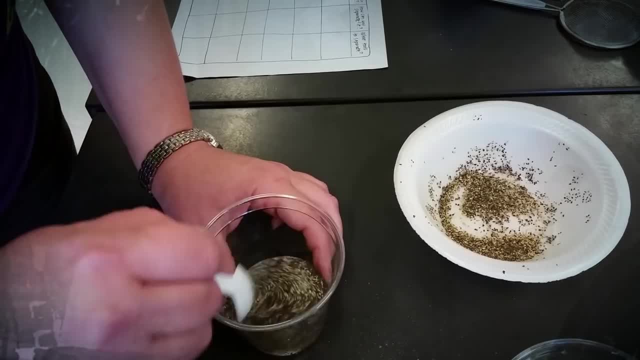 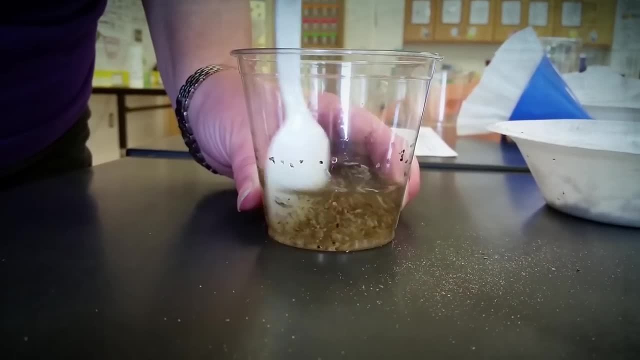 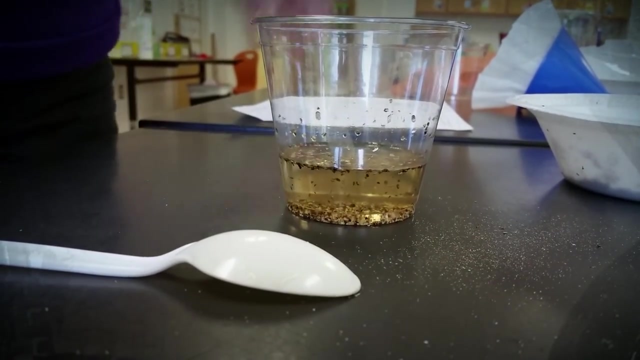 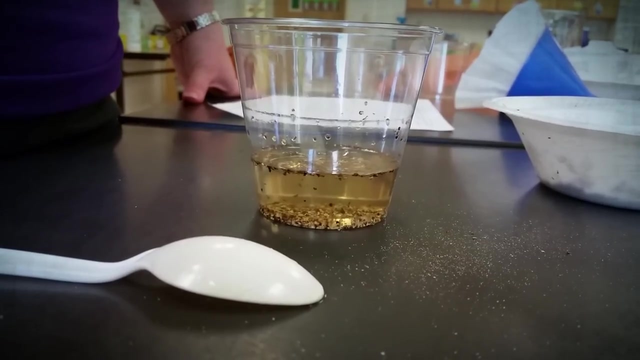 in your describe the mixture column and I want to stir and get that pepper all mixed in there. okay, you can see some of its floating, some of its sunk to the bottom, so it's all throughout the water, okay for our. did the properties change column? so did the pepper change did? 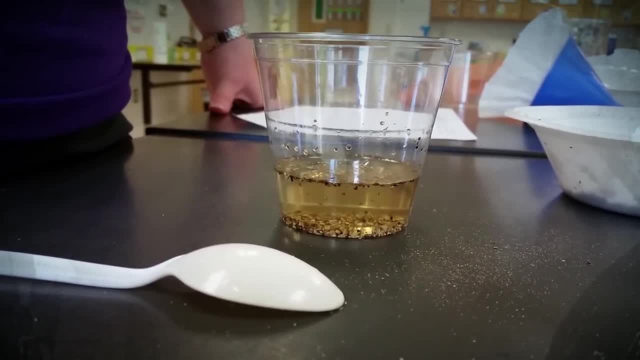 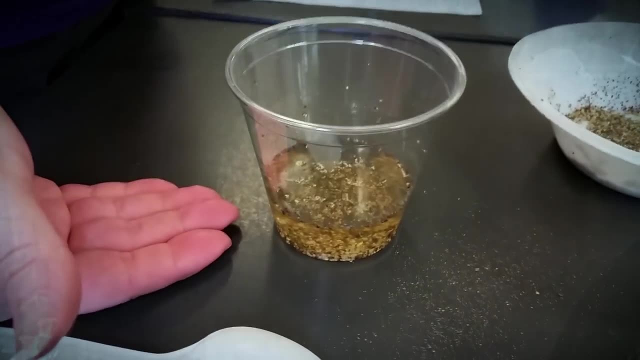 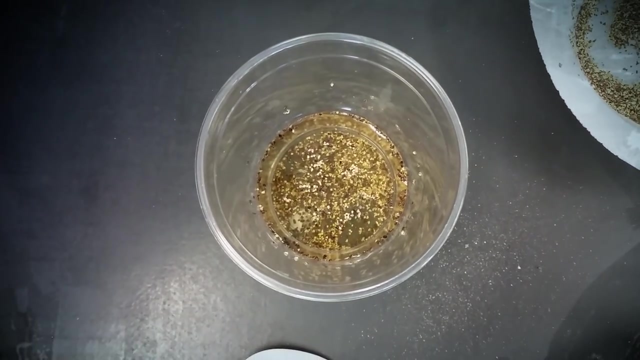 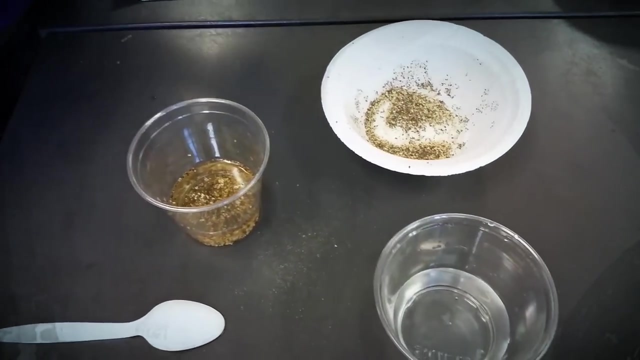 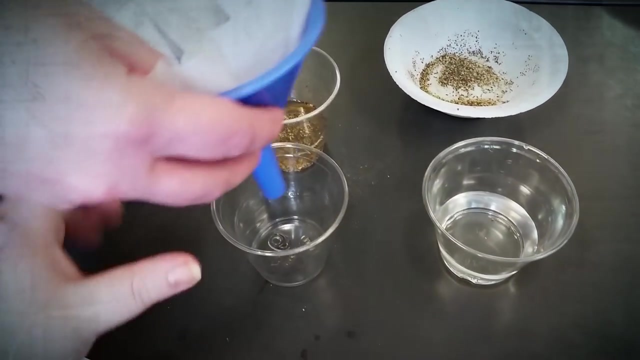 it dissolve into the water, yes or no? for our mixture or solution so is if this dissolved, it would be a solution. so if is it a mixture or is it a solution? now we're going to separate it. so how can we do this? okay, I have another cup and we're going to bring back our filter and our funnel. I'm going to go ahead and 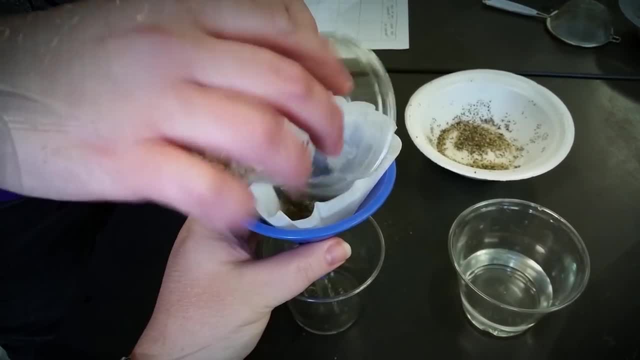 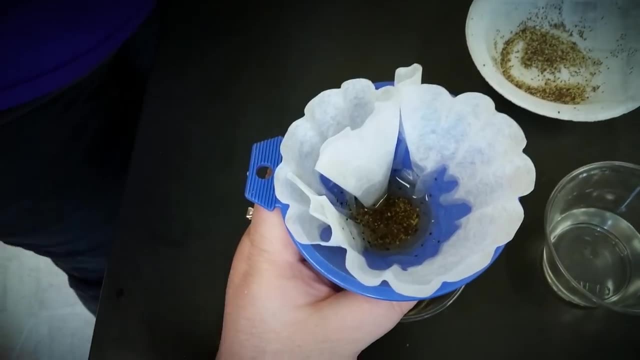 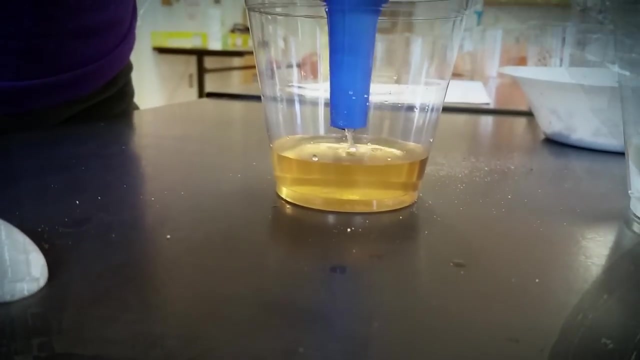 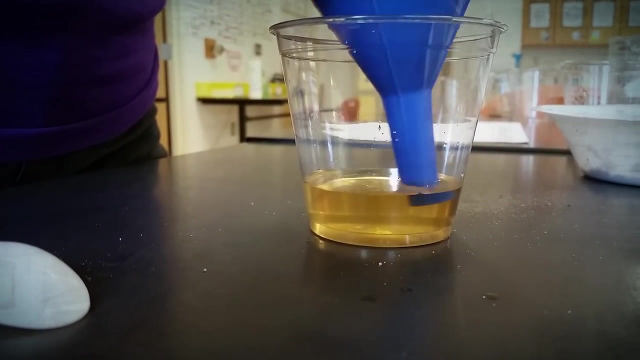 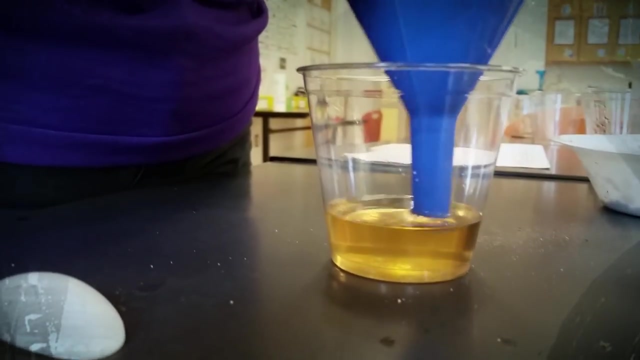 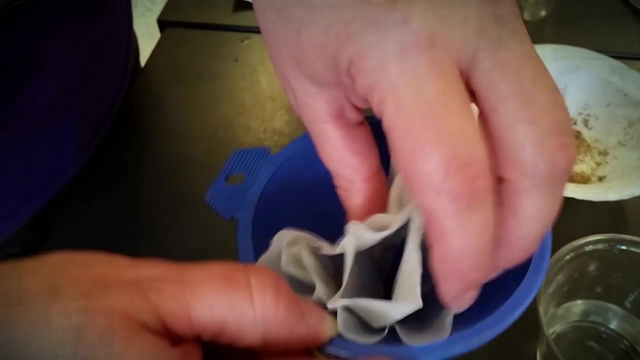 pour this in and you can hear the water draining through the filter, through the funnel. this minute got a lot of water there, okay, so I'm gonna pull the filter out and we can see that here's all of our pepper captured in the filter and all of our water has gone through and into the cup again. now you notice our water. 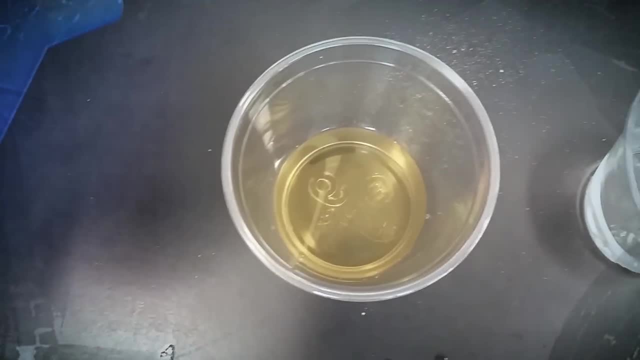 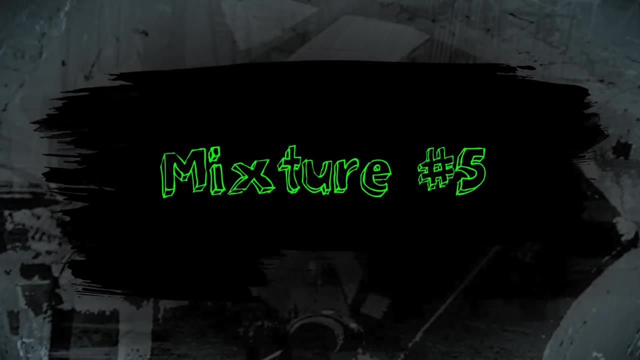 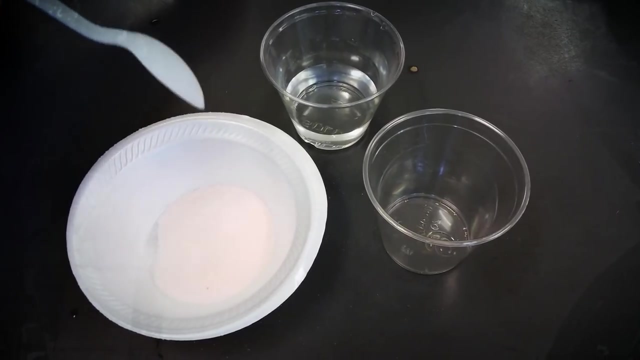 is a little darker than we started because that pepper kind of changed the color, but there's no pepper flakes in there, so they got captured in the filter. there's no pepper flakes in there, so they got captured in the filter. all right, we should now be on the fifth row. I am going to look for another solid and liquid, so I 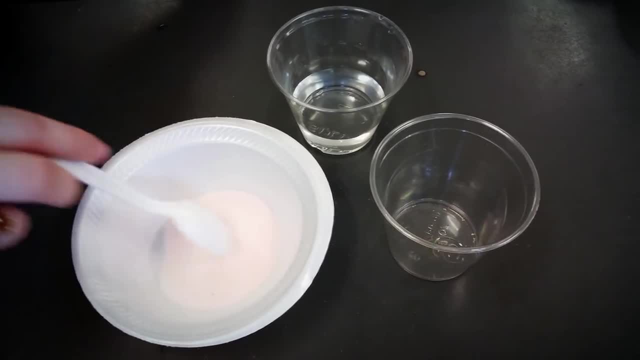 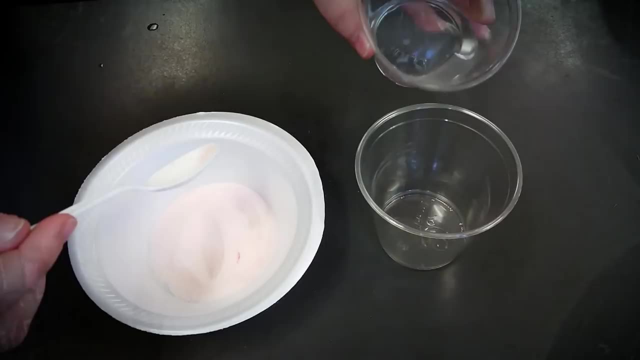 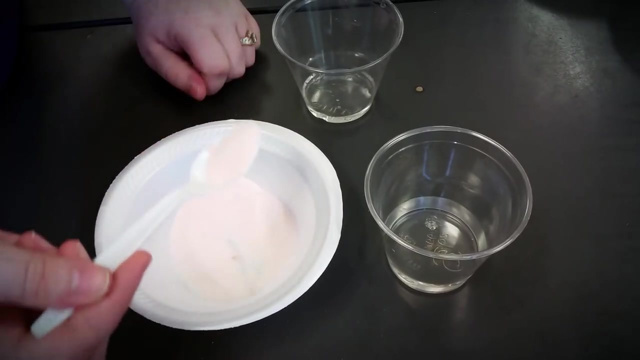 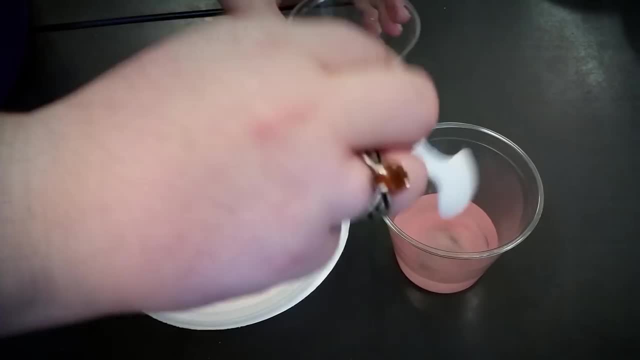 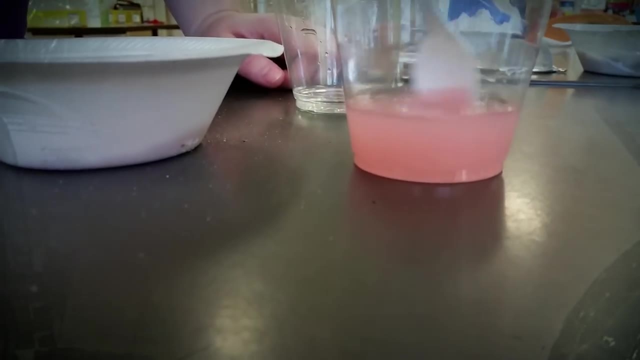 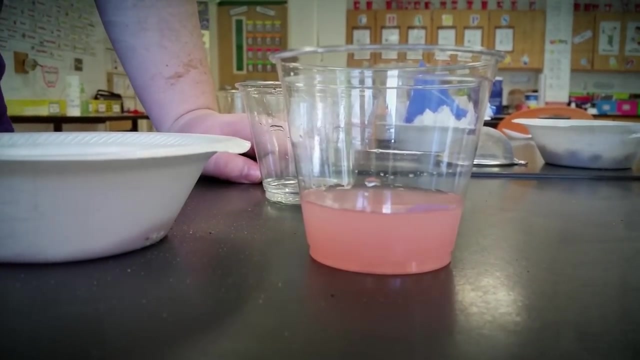 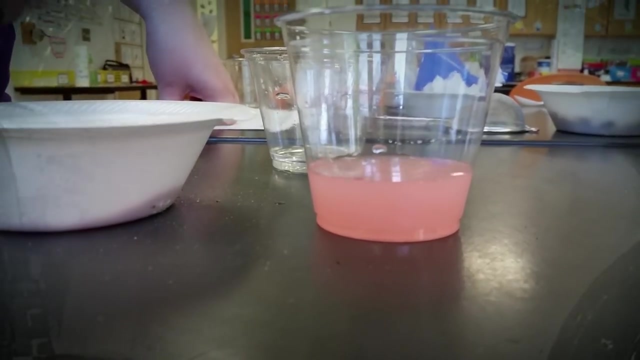 and a little bit of water of pink Kool-Aid mix. I don't have a whole lot of water, so I'm just gonna put a little bit. mix it together. You may see that the pink color is the same throughout. it's not really settling. it's pink the whole way through. 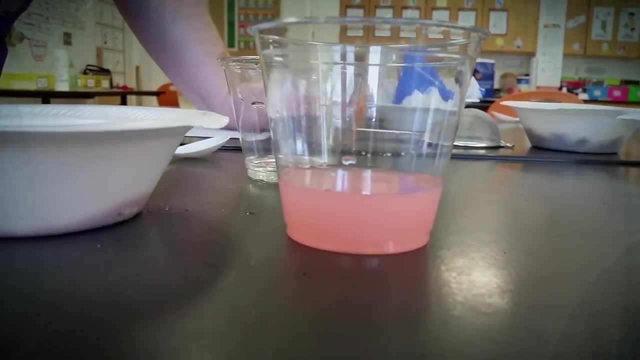 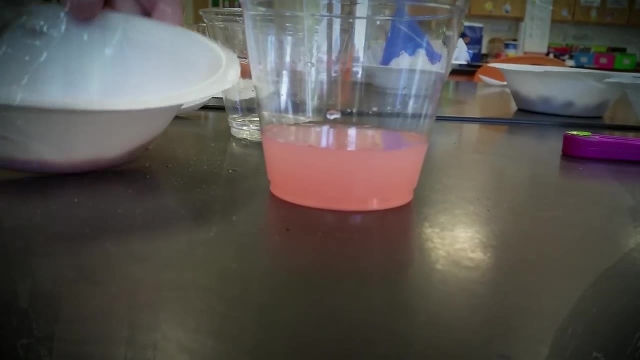 Now if I were to take something like a magnet to this, it's not gonna work, nothing's gonna move, Strainer's not going to get these itty bitty pieces of stuff out, So I'm once again gonna use my funnel. 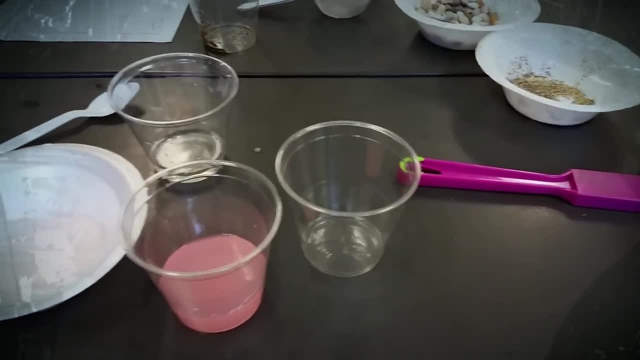 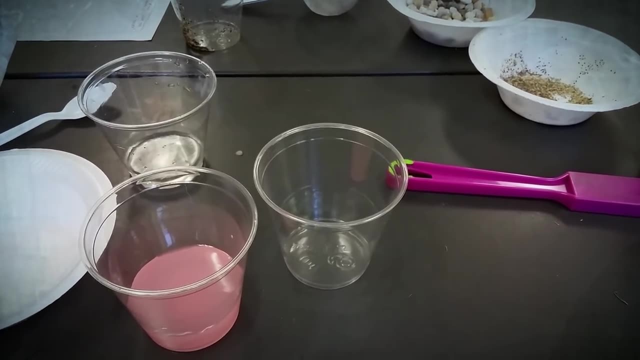 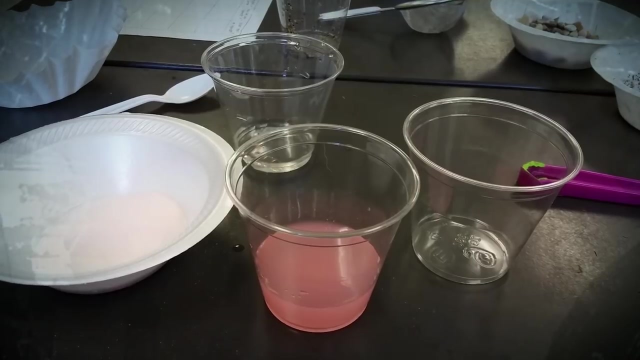 And I have a second box And we are going to decide while I am putting this funnel on here. did the properties fit? Is it gonna change? Is it a mixture or a solution? And we're going to try and separate it with a funnel. 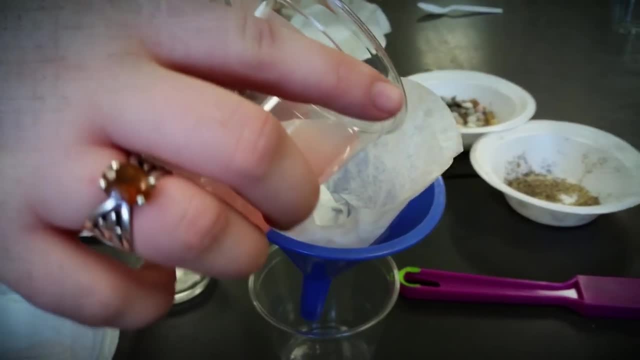 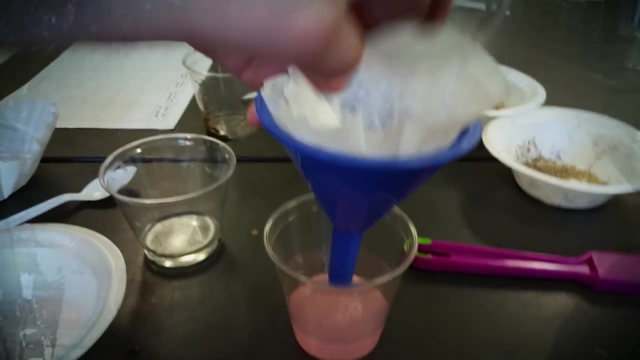 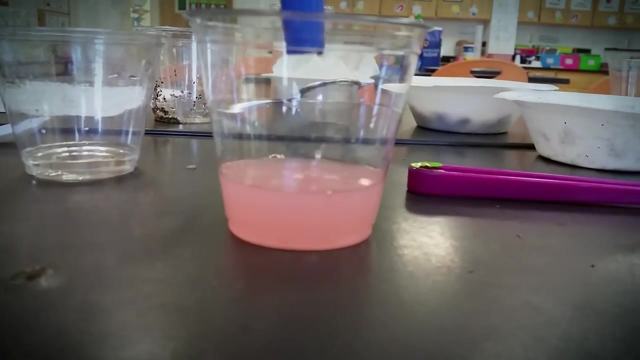 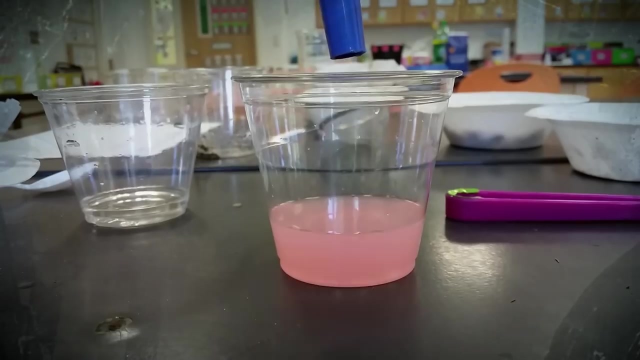 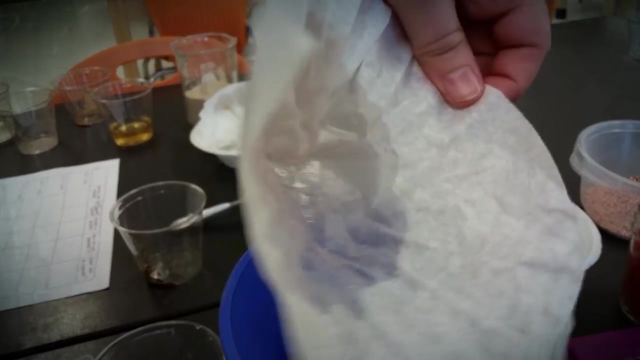 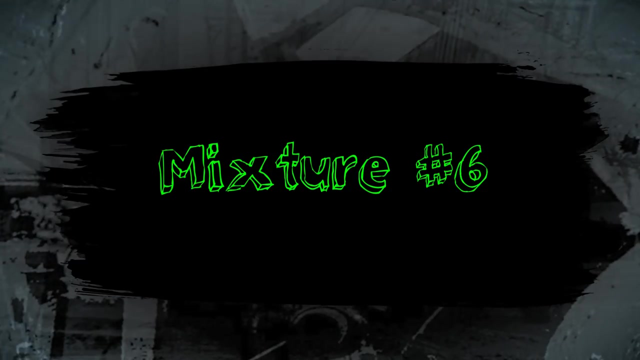 See if it works. Look, the color that's coming through is actually pink, So I want you to decide as a class now separating it. if it's coming back through as pink inside my funnel, you'll see that I don't have anything except for a little bit of moisture. okay, for. 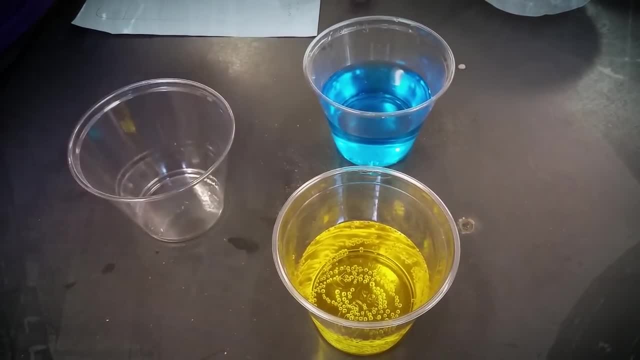 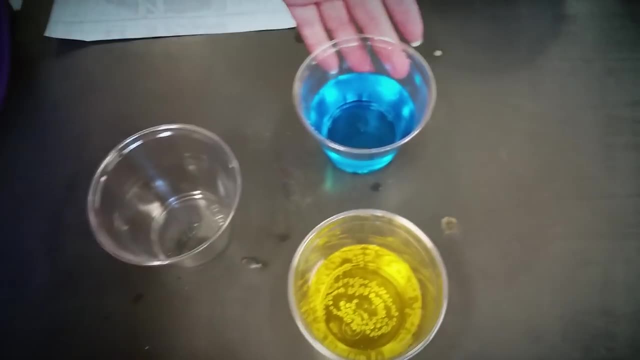 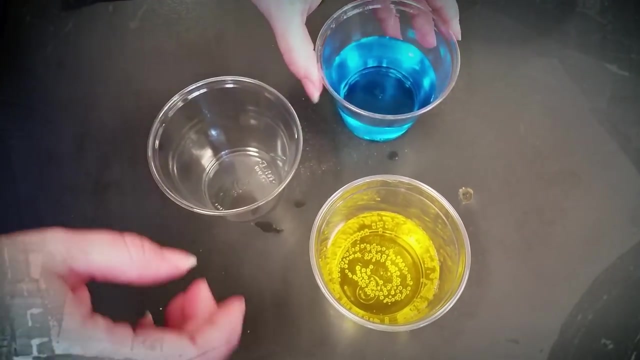 your bottom row it says liquid plus a liquid. so right here we had two clear liquids. so we put coloring in them so that you could see the difference. the water we put the blue food coloring, and then this is sprite. so we put some yellow in here. so we're going to pour a little bit of both into this empty cup. 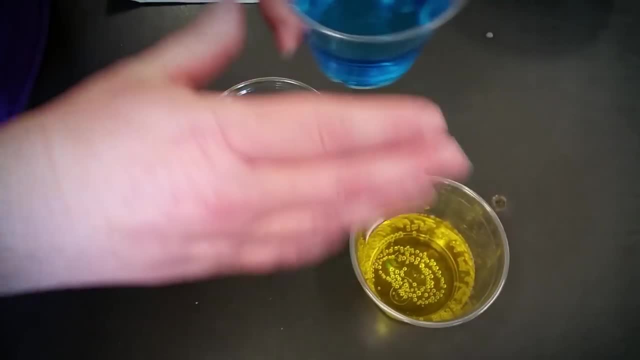 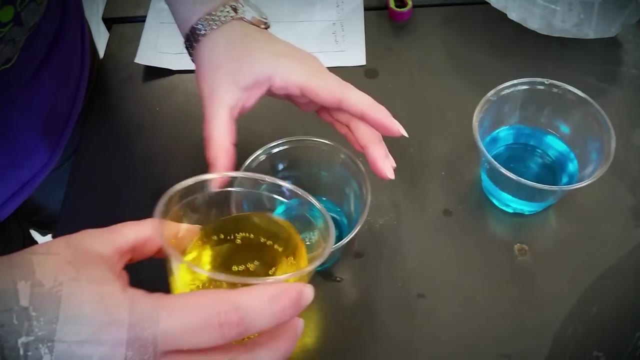 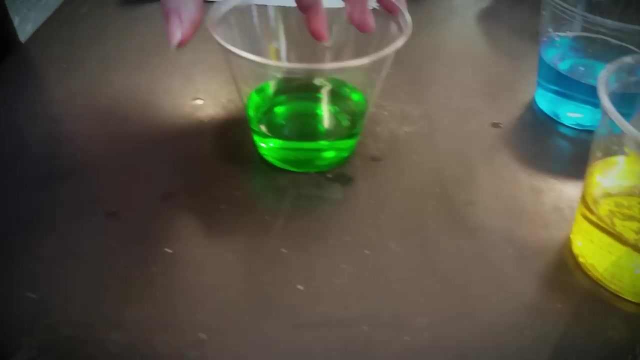 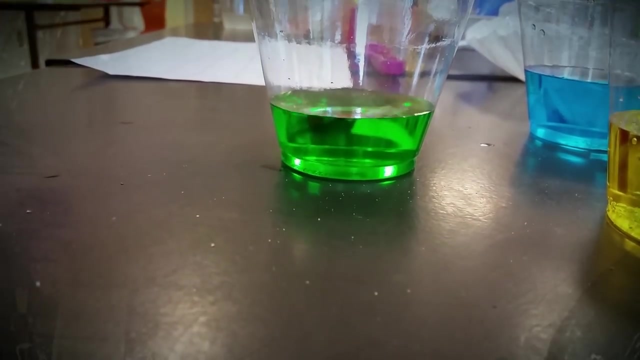 so go ahead and write both of those down: water and sprite on your describe the mixture column. ooh, the pretty color change. now we have the green mixture, which is both of them. so we need to decide: is it a mixture or is it actually a solution? so we don't see any particles floating. 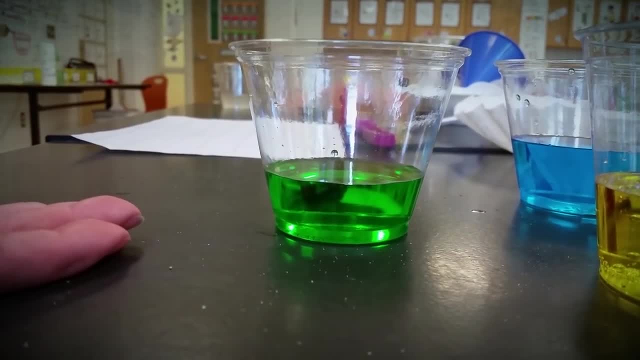 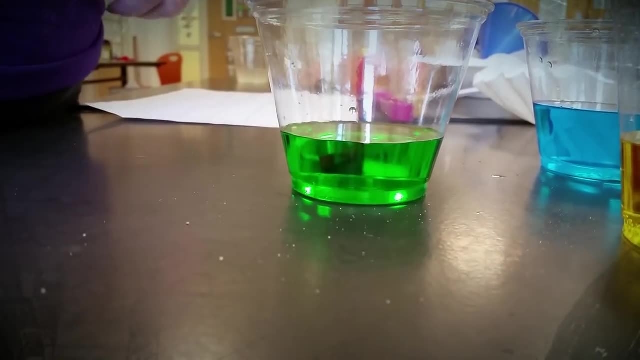 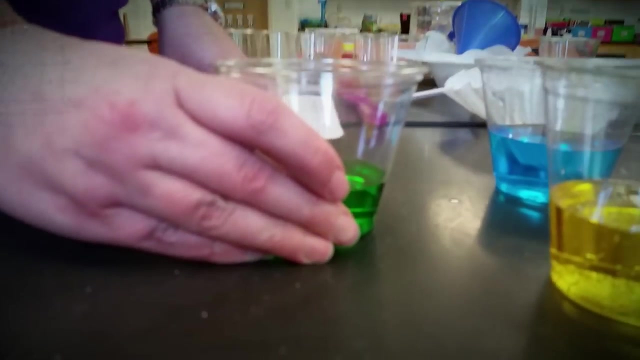 around you can't see any difference in the liquid other than the color. so did these properties change from water and from Sprite? so now we're going to see if we can separate the two back to water and back to Sprite. so I'm going to try a magnet. nothing sticks to. 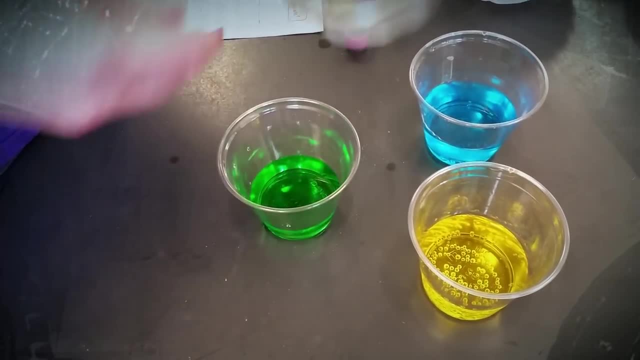 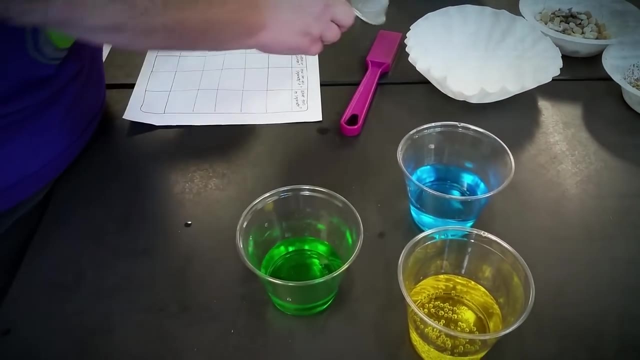 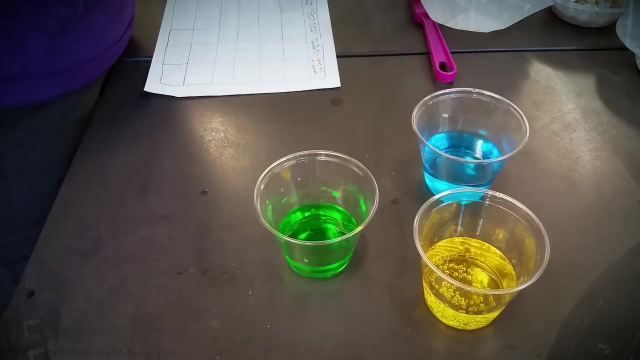 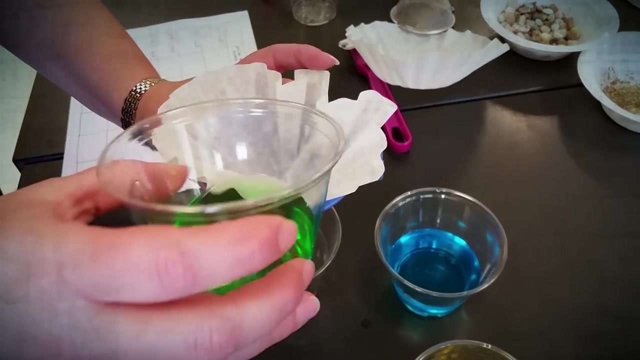 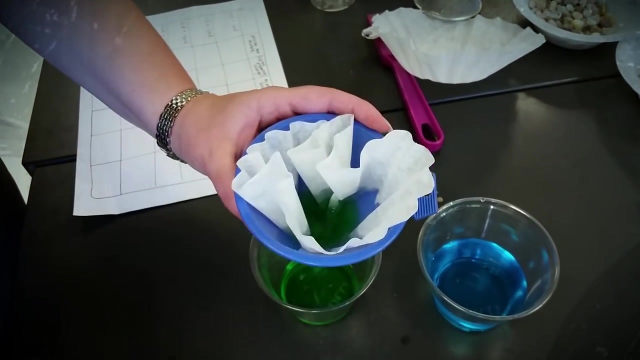 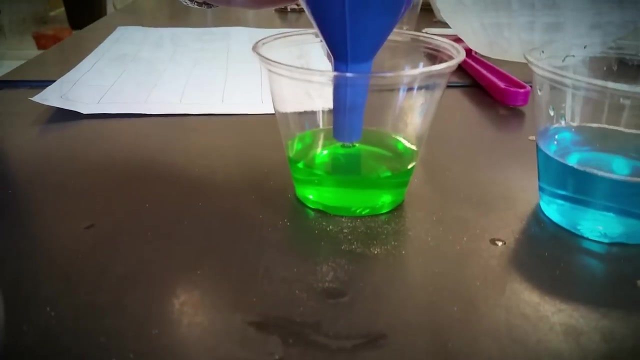 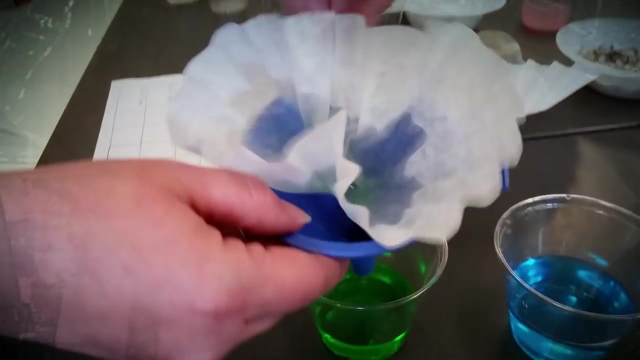 that if I use the sieve, all liquid would go straight through, so that's not going to work for me. so let me try my filter again with the funnel. another empty cup. okay, so pour our green liquid in. everything's straining through. ok, we can see the filter is moist from the liquid, but other than that there's. 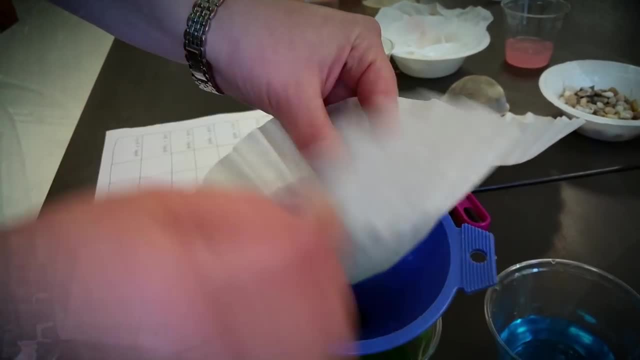 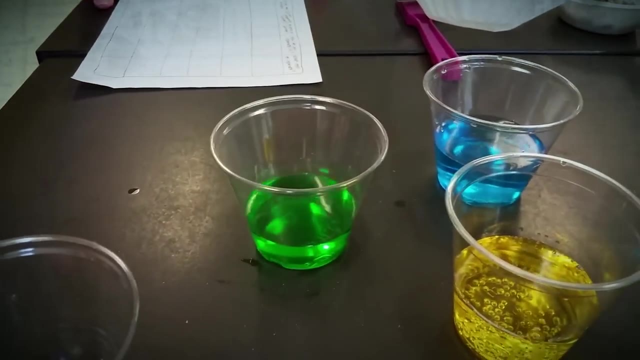 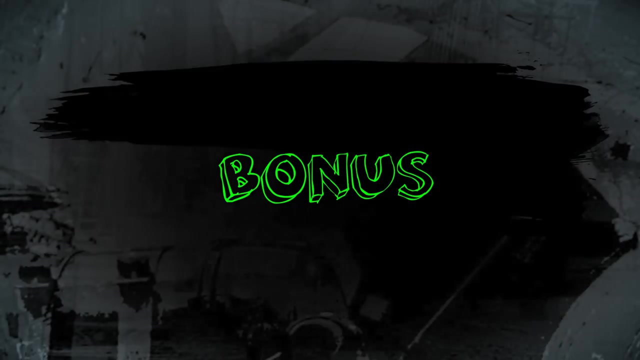 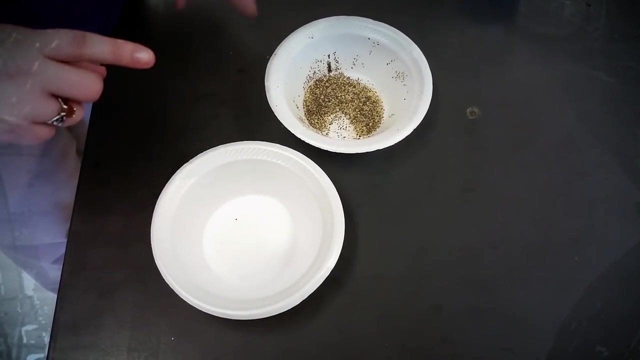 nothing really left in. it didn't capture any water and we still have all our green liquids, so we can't separate them. so what does that make it? a mixture or solution for our first bonus activity? we're actually going to use two solids and later we'll join a liquid in. our first solid is: 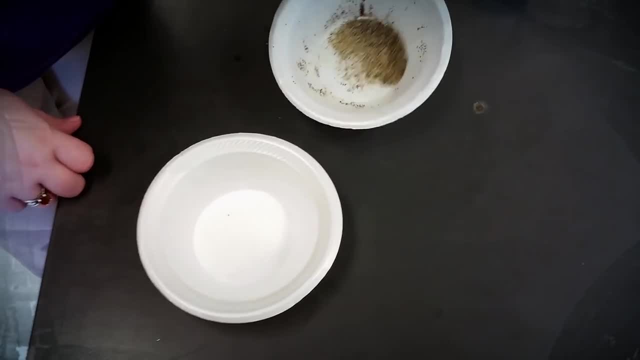 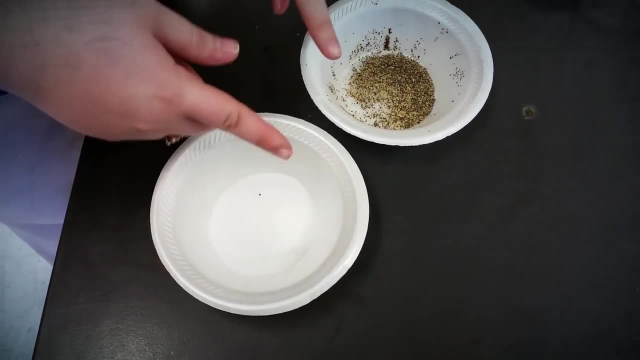 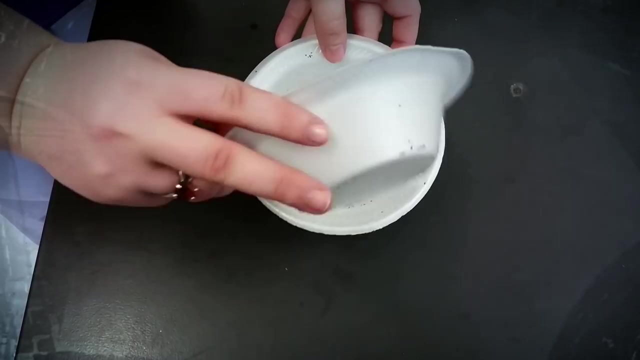 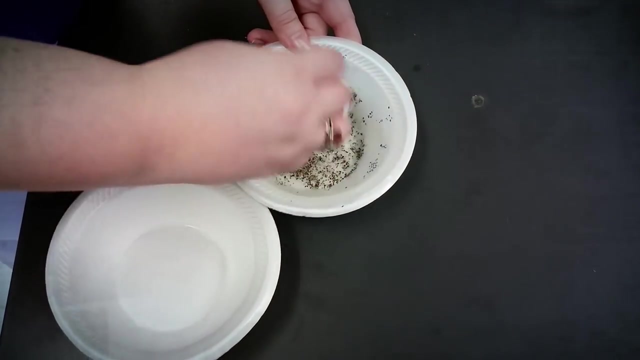 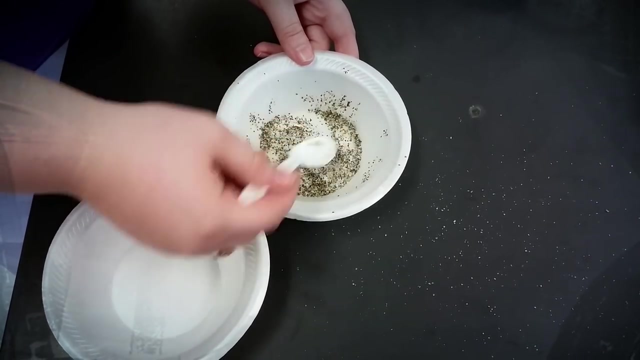 pepper. you can see it is in solid particles. we move around individually. second one is salt. I am going to go ahead and I'm just going to mix them together. we don't need them after this, so here we go. it is all blended together. I just made a mess, it happens. you can see that it is all blended together. 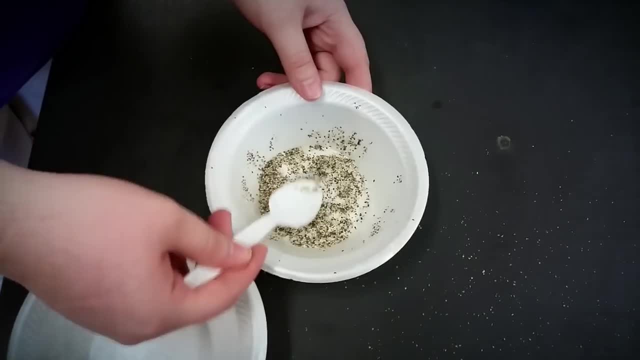 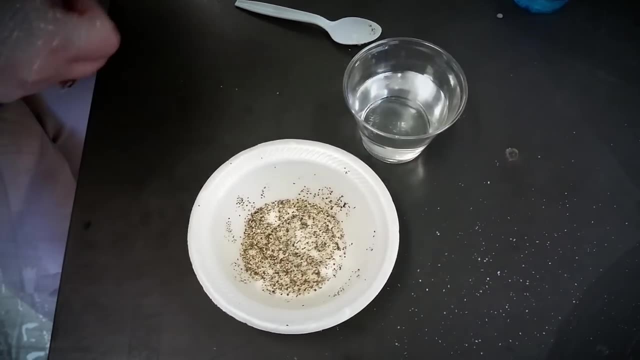 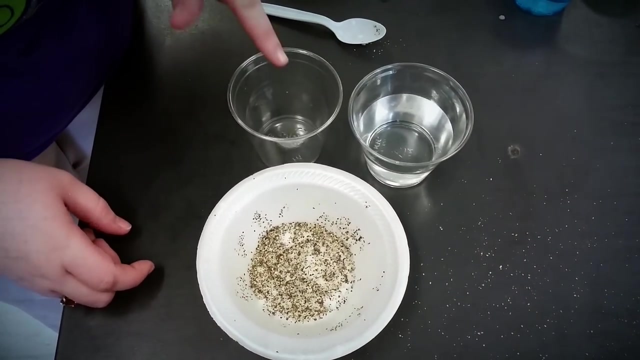 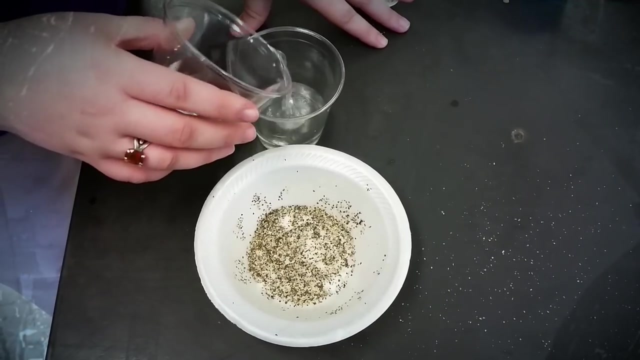 now, over here, I have my water. now that we have our pepper, salt and water, I'm going to actually combine them into this third container, so I'm going to put a little bit of water. while I'm doing this, I want you to be thinking to yourself. 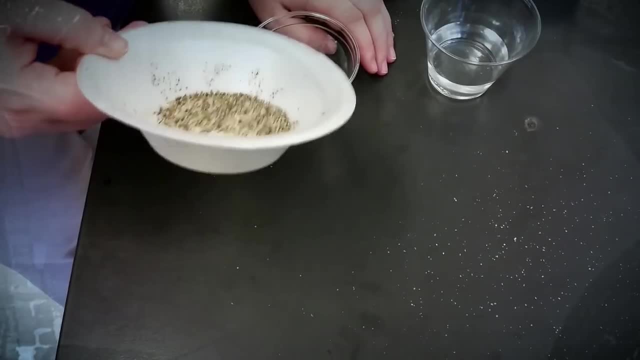 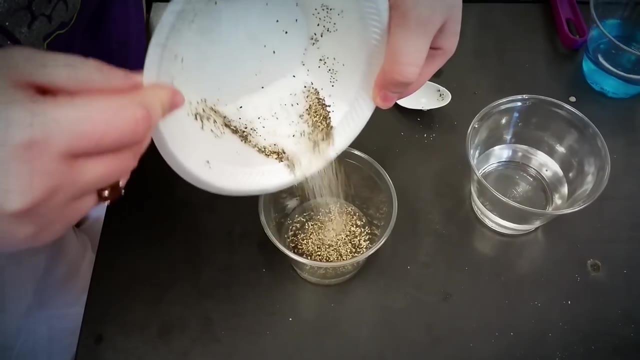 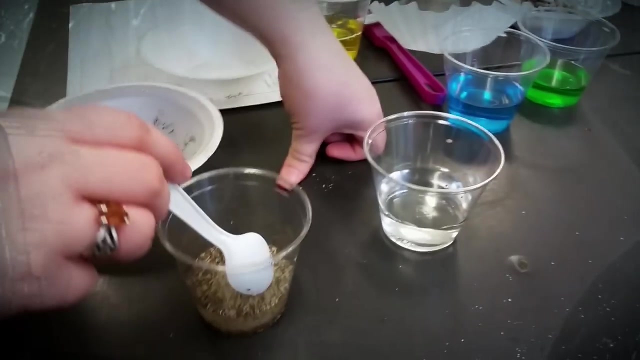 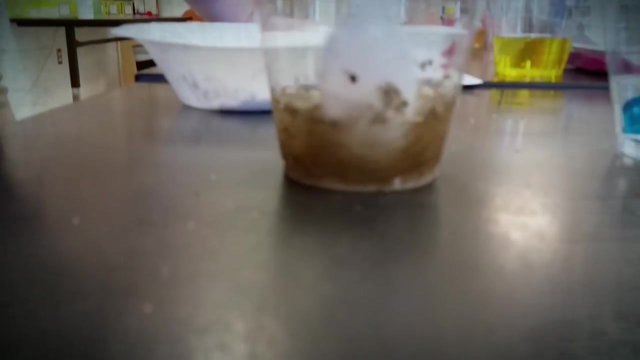 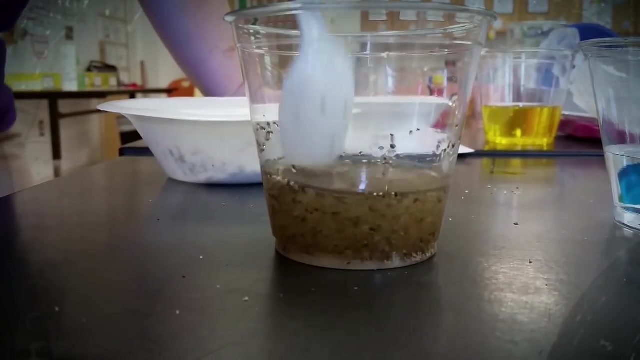 how are we going to be separating the salt and the pepper from this liquid and just gonna live on the edge, put quite a bit in there. you may see, like we saw before, that the pepper seems to be still in chunks. it's pretty separated from everything. you see some at the 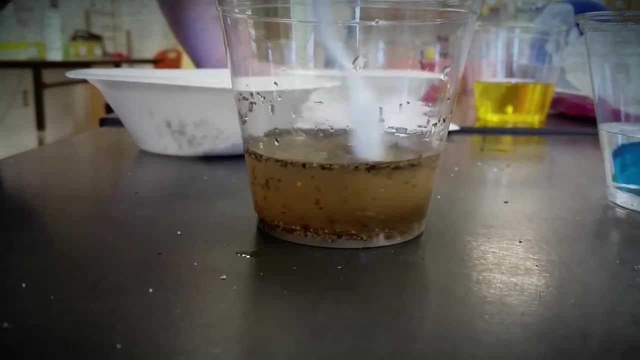 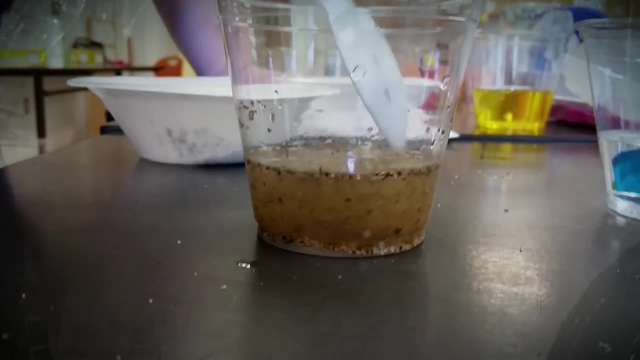 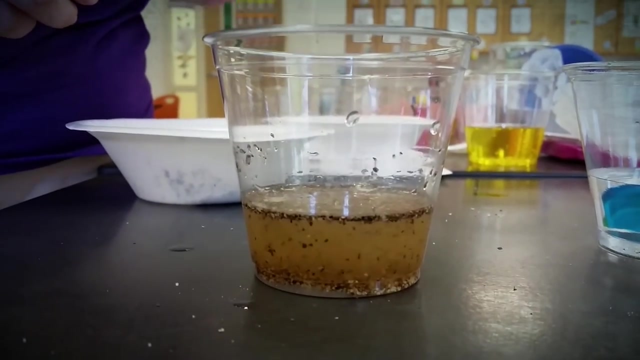 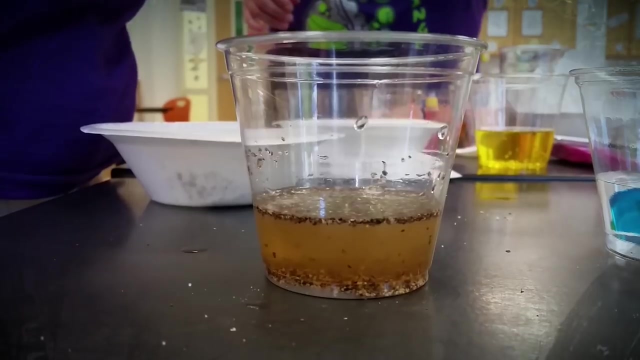 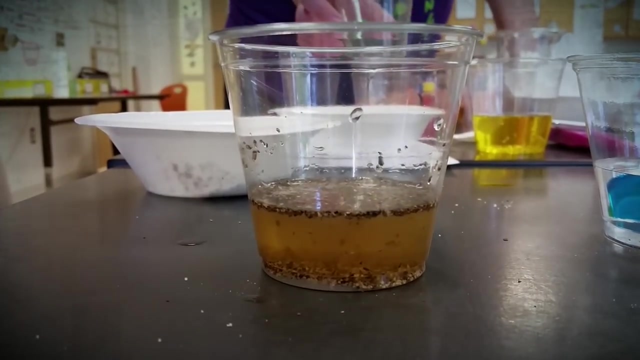 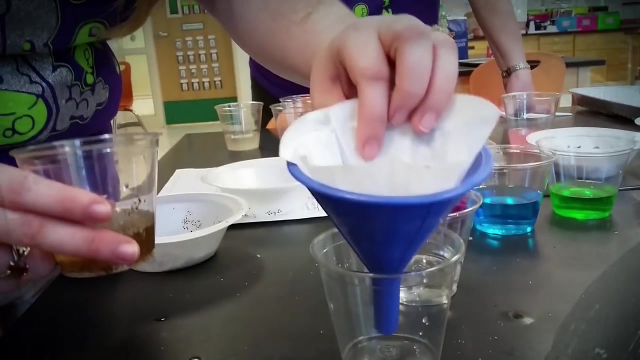 bottom and some at the top. the salt, on the other hand, is starting to dissolve, as we talked about earlier. when things dissolve, we call them a solution. okay, I am going to try and separate out my salt and pepper by using a funnel, because we found earlier that worked with the pepper. pour it in here. 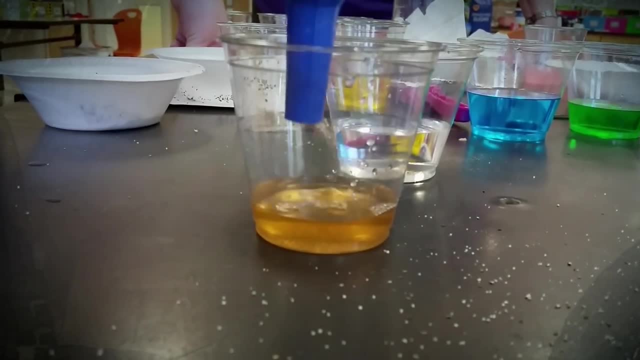 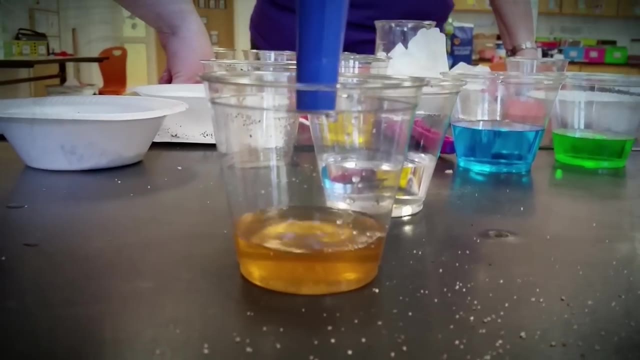 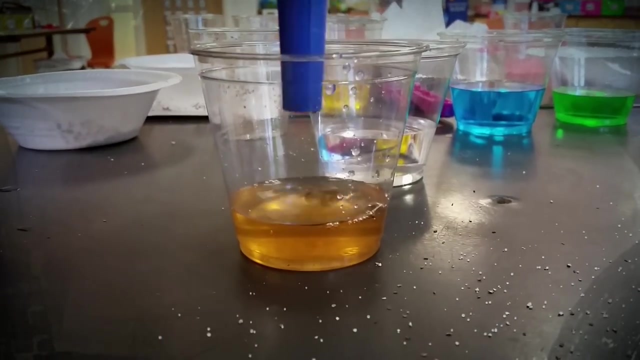 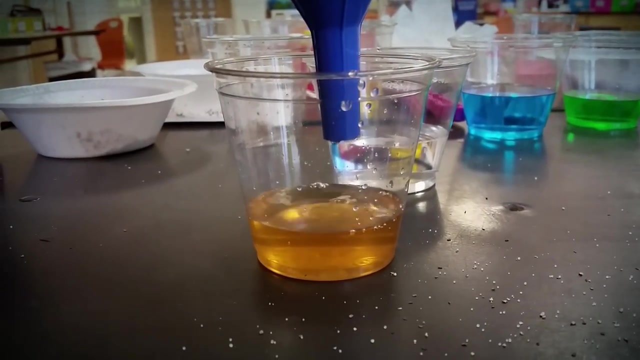 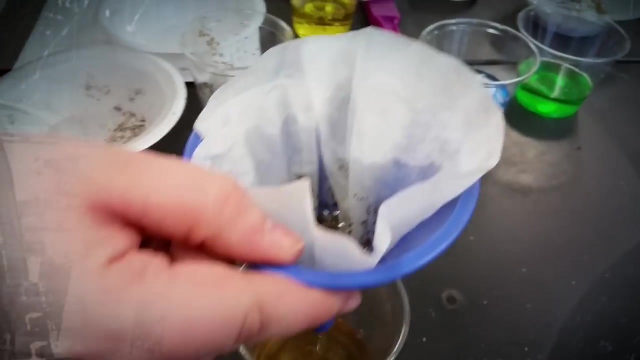 you can see, like before, that the pepper kind of stains the water color, sort of like tea leaves. but I don't have any pepper chunks down in my bowl. we're still filtering. see if I can speed it along here. we're still dripping, but you can see on the top part that I have a little bit. 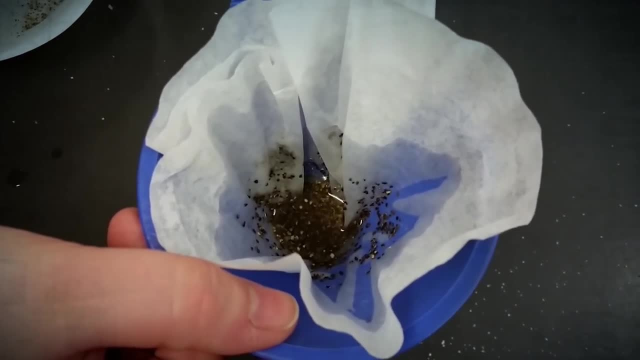 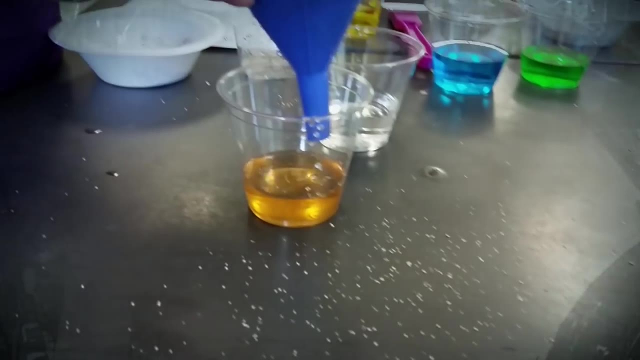 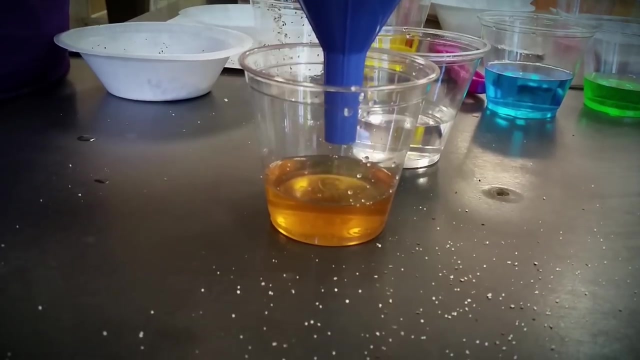 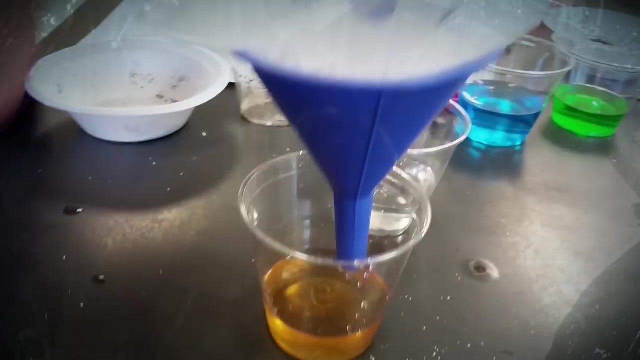 of salt in there. I just need to pour it in there for the next few seconds. I'm just going to go ahead and pour it in and see if I can get it to that consistency. we're still dripping, but you can see on the top part that I have a little bit of 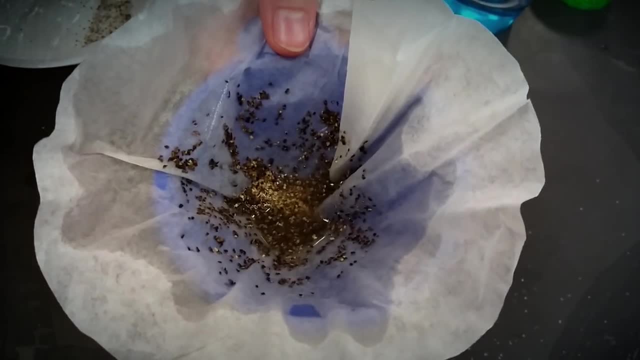 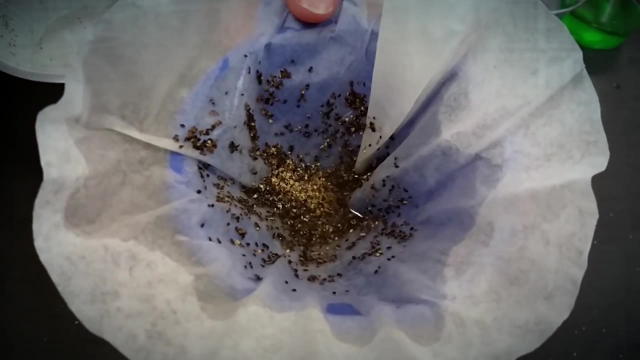 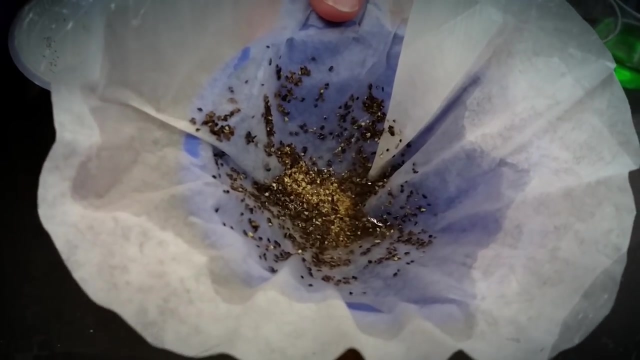 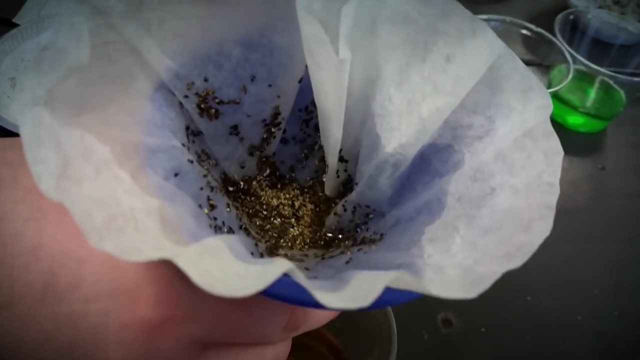 have pepper flakes in the top. The water is almost completely dripped through, But I don't really see any salt in my filter. So now we're going to have to try and find a different way to get the salt out of the water, because that part is a solution And, as we saw before, 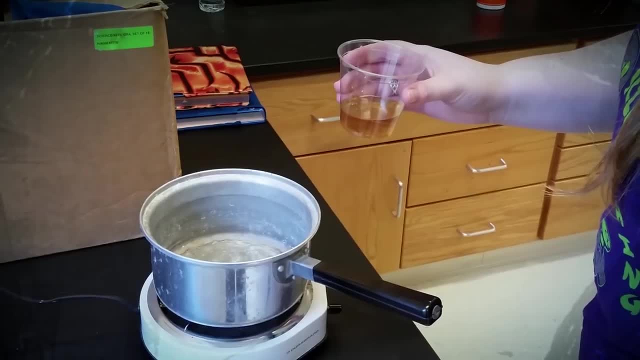 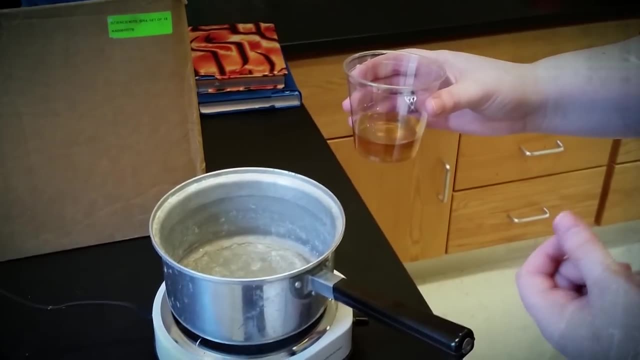 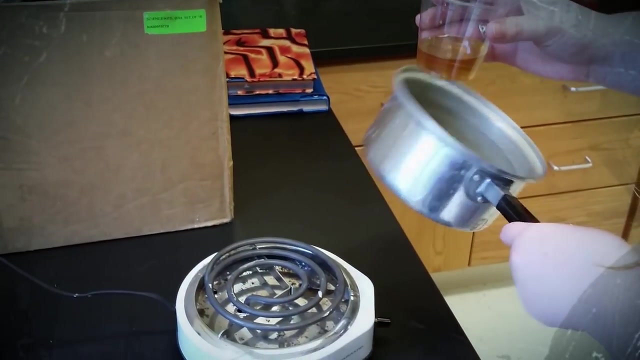 filters do not work on solutions. Okay, when the filter doesn't work and the magnet doesn't work and the sieve does not work, we have to find a different way to separate out our solution. Science uses heat a lot, So here we have a burner. It has heat coming off of. 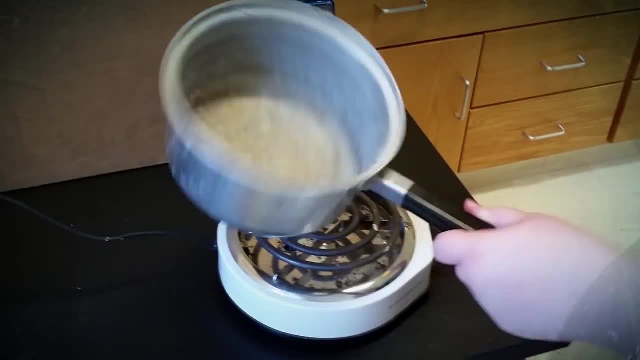 it Very hot And I have a pot pan. I'm going to take my solution: I'm going to pour it in here and we're going to wash it, And then I'm going to pour it in here and we're going to wash it, And then I'm going to pour it in here and we're going to wash it, And then 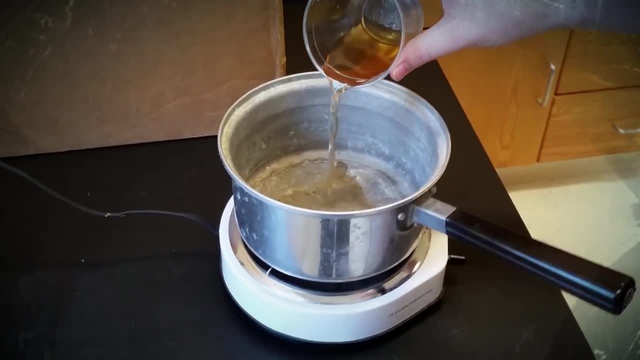 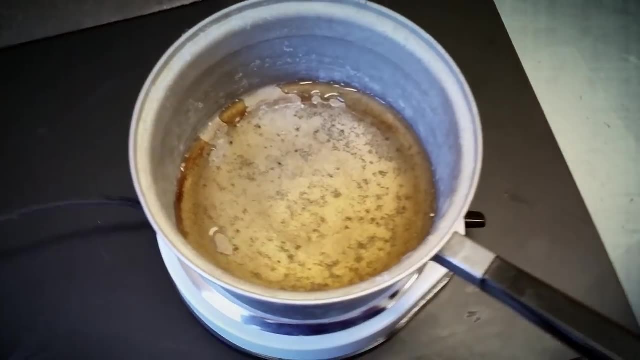 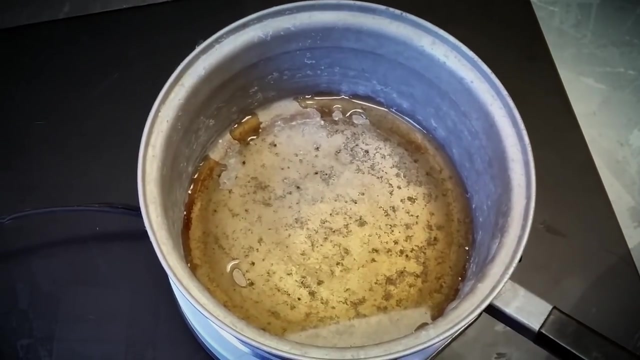 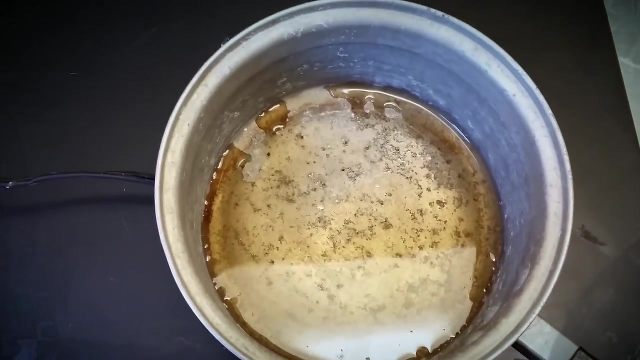 we're going to wash it And then we're going to watch what happens. So, as the heat is being applied to this pan, we know that water is going to begin to heat up. And as it hits 100 degrees Celsius, what is going to happen? That's right: The water is going to evaporate. 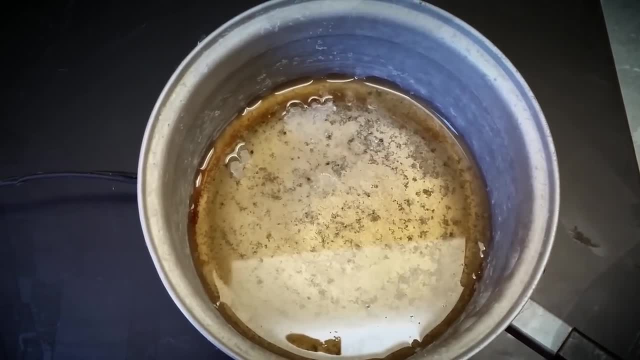 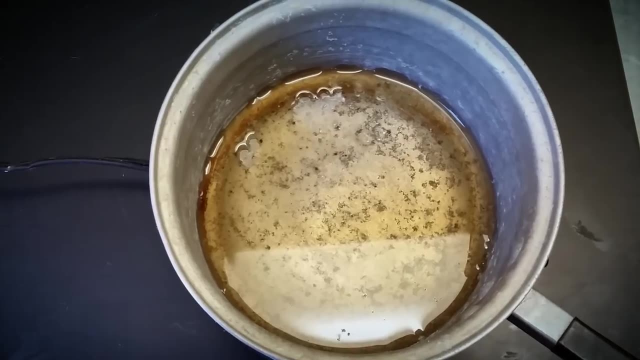 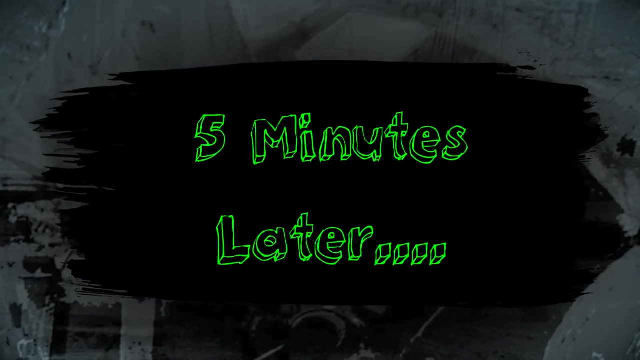 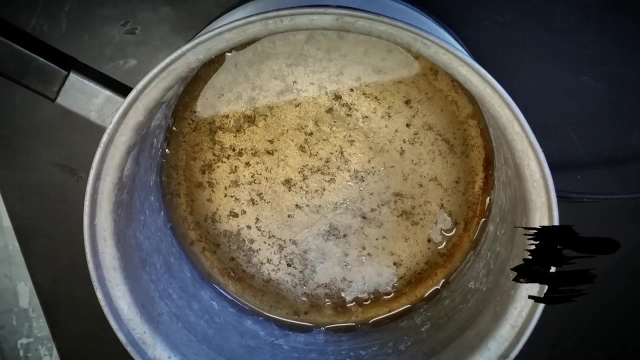 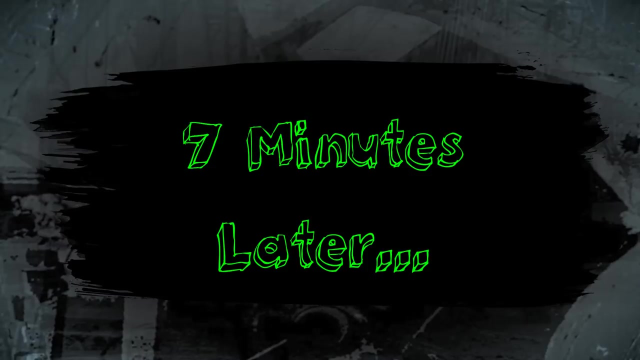 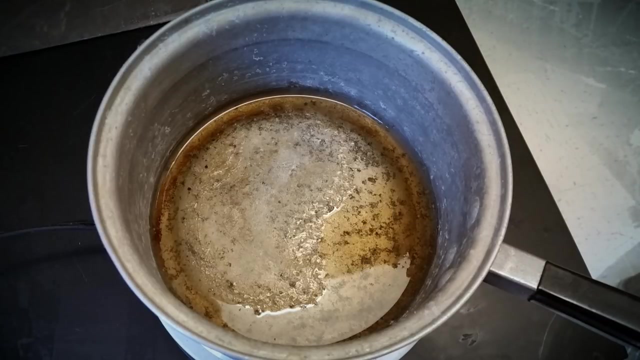 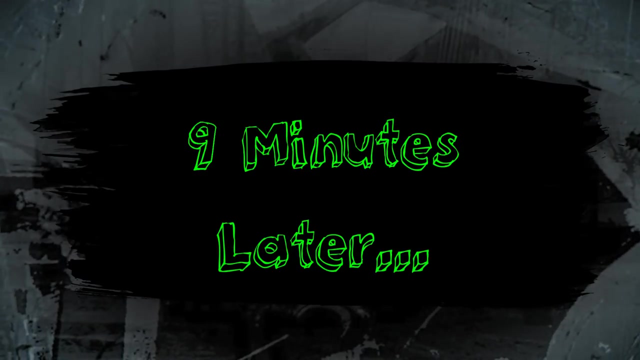 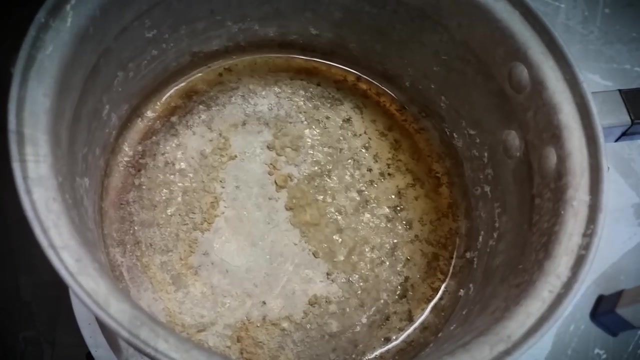 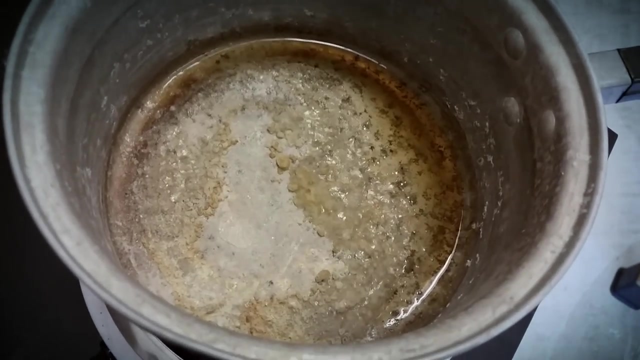 And when it evaporates it turns into a gas. What we're going to have left is going to be our salt. All right, We've had a little bit more time pass And as you look closely, you can see that now we have some very large salt crystals starting to form. 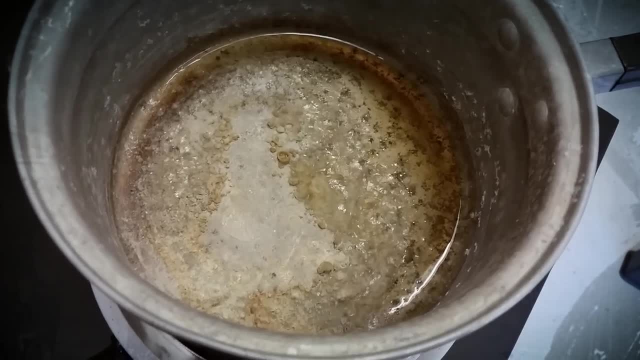 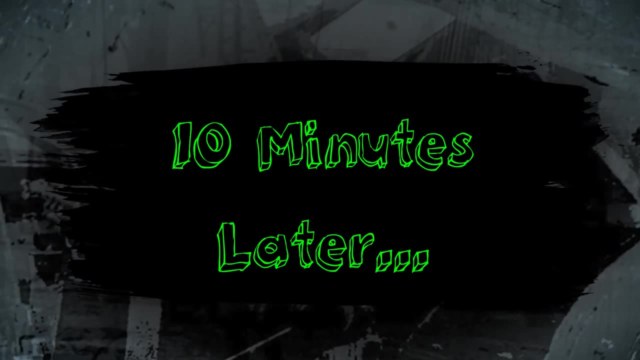 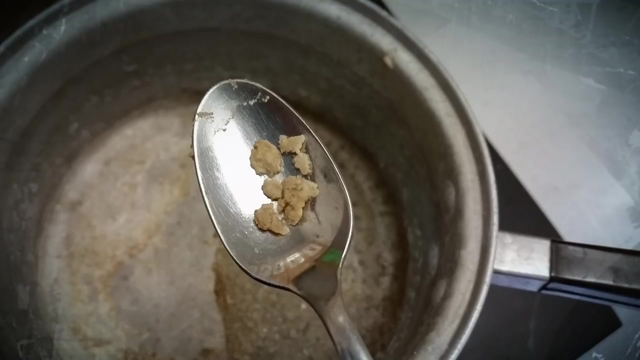 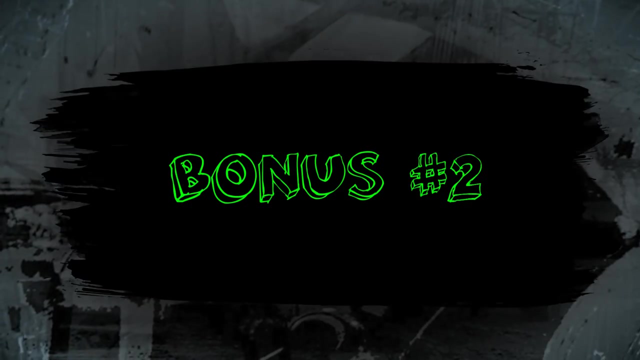 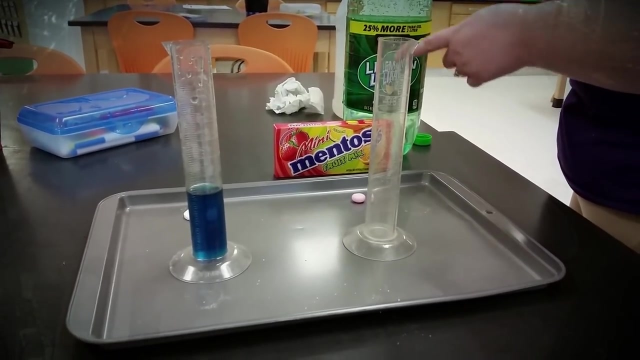 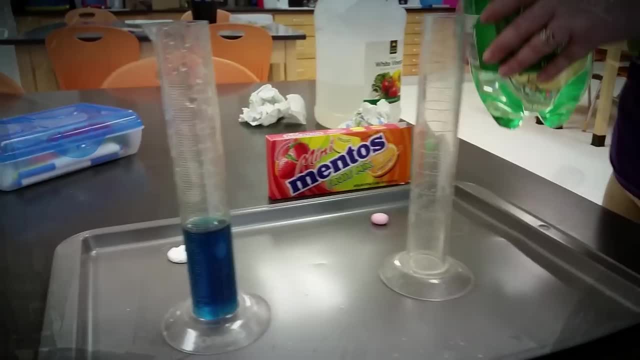 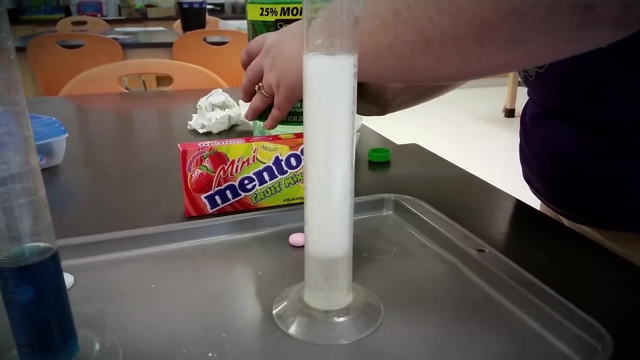 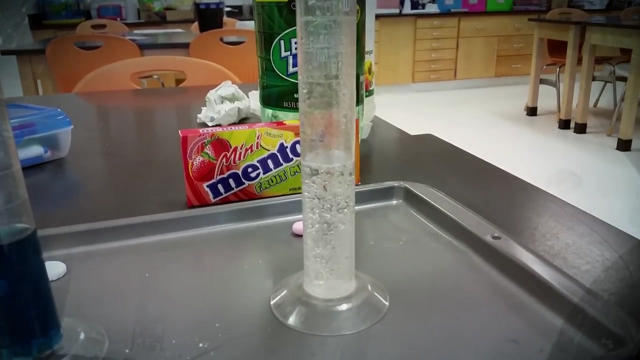 I'm going to pour the soda in there. When we first pour it in, it's coming out of the bottle and you're going to see that it's already got some natural carbonation. We're going to let those bubbles die down just a little bit. You'll see that the liquid is more calm. 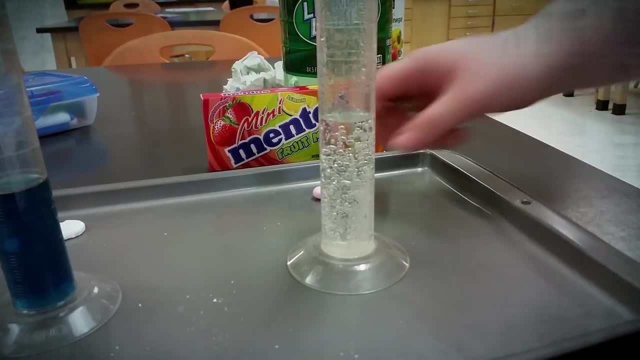 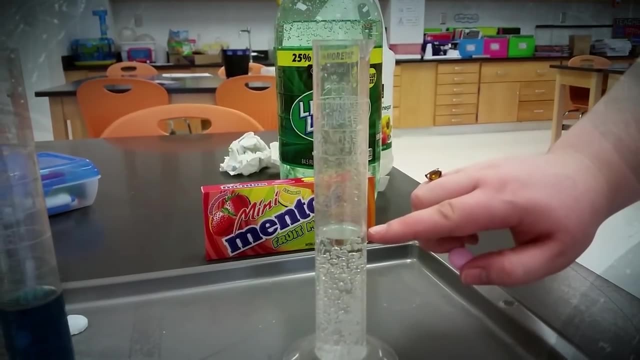 We do have a few bubbles on the side. It's a soda, so you're going to have some carbonation. I'm going to take a Mentos and you'll see. the water is right here and we're going to watch what happens. 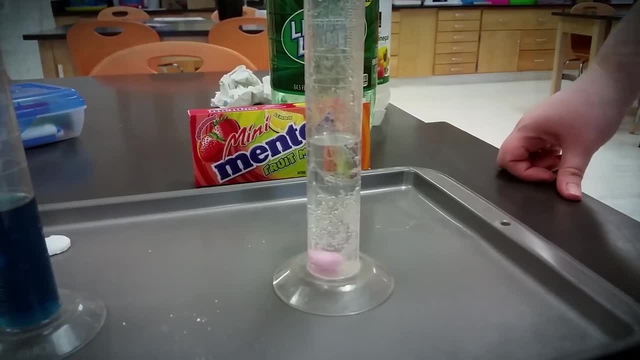 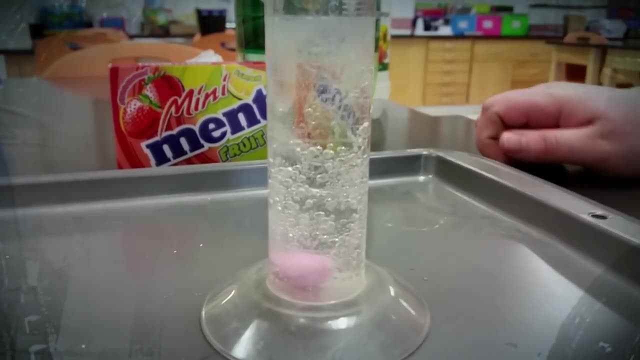 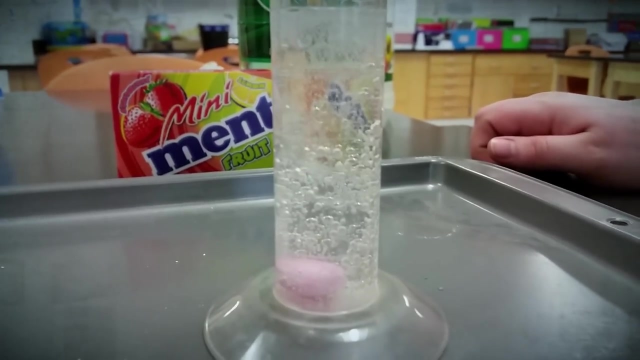 Three, two, one. As you watch, you're going to see that you have a cloud of tiny little bubbles that look a little different than the carbonation. That is the Sprite going into the pores of the Mentos. and as it goes into the pores, 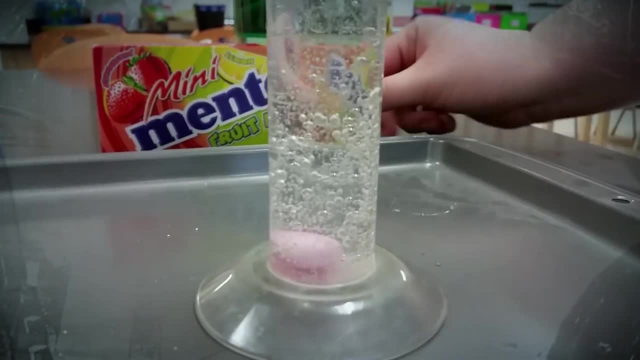 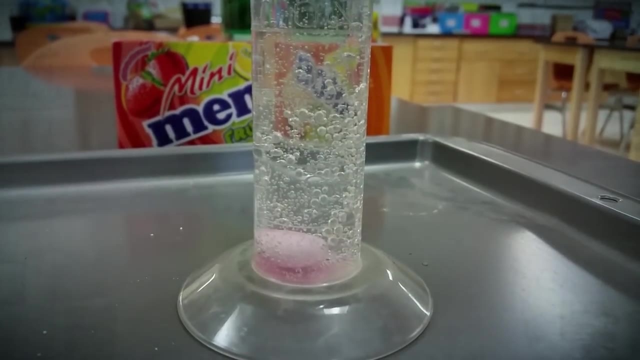 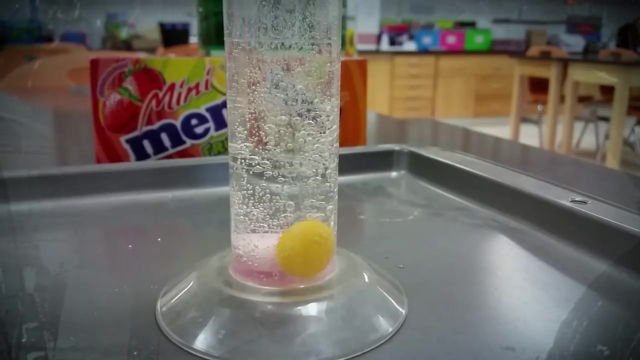 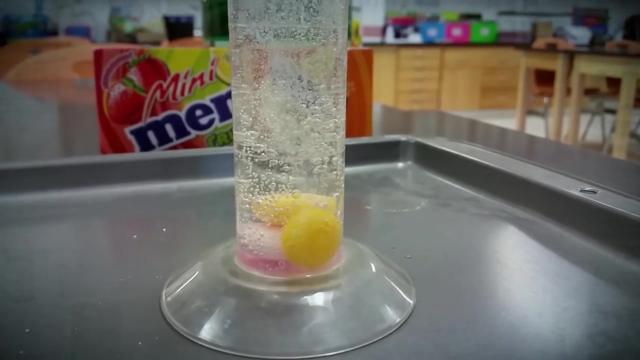 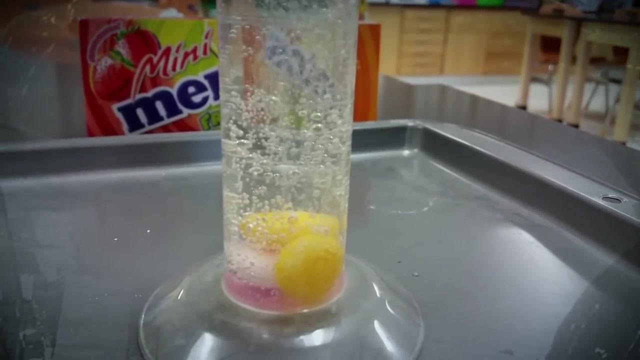 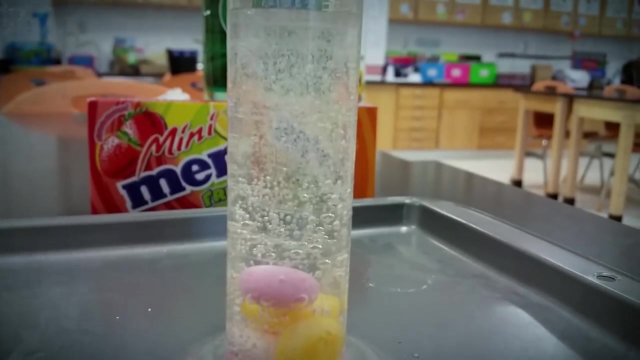 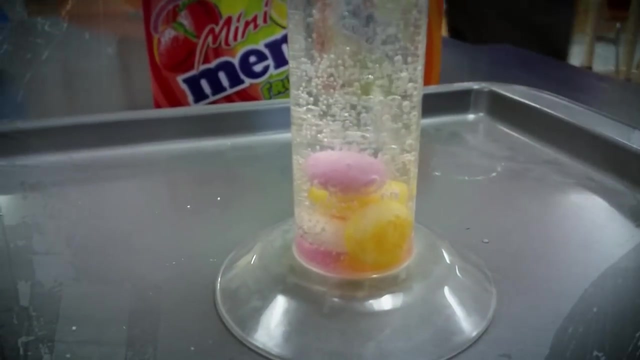 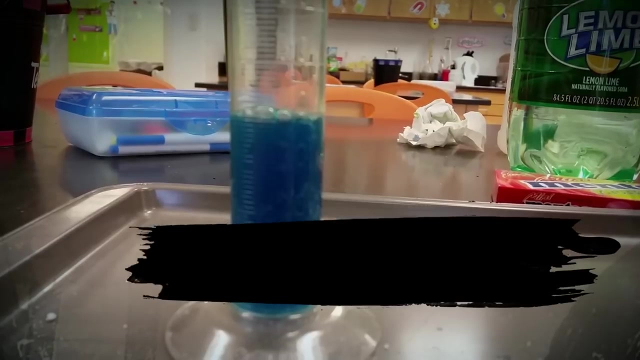 it starts to build up more gas, which is released. I'm going to go ahead and add some more and you'll see another little cloud start to form. Okay, And that is our Mentos and Sprite experiment. Okay, and for our final experiment, we have some vinegar colored with blue food coloring.